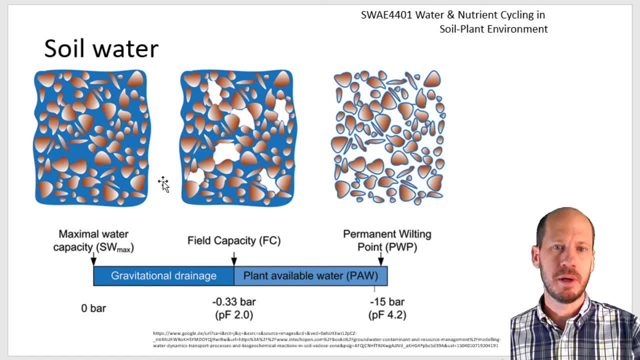 talking about soil water and soil water availability to plants. plants need to absorb quite a bit of water. the crops need quite a bit of water from the soil, and we were talking about how are the the, what are the factors that condition the availability of water to the soil? and we saw some key concepts like field. 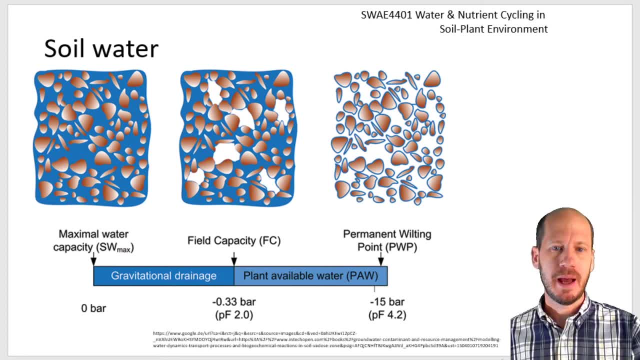 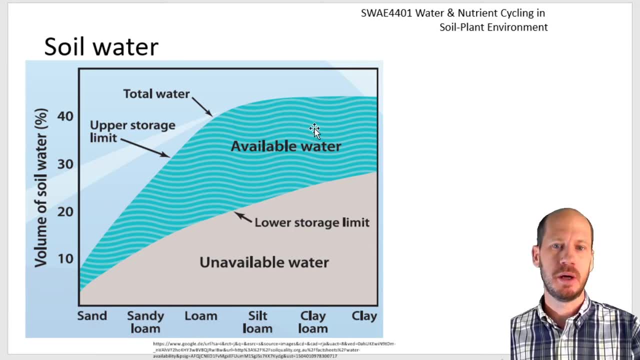 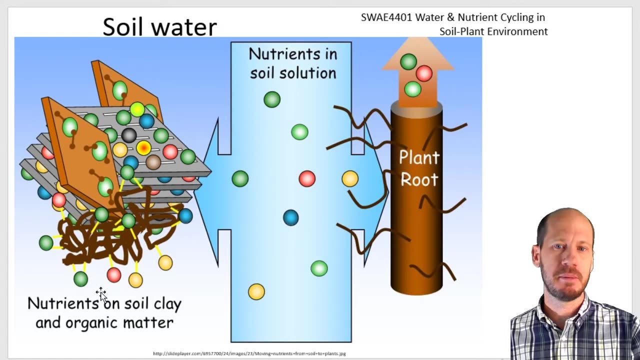 capacity and permanent wilting point, and how this field- capacity and permanent wilting point- varies with different textures in a conditioning, the amount of available water present in different soils. but today we're going to move on from that, those concepts, and we're going to start talking about what is the interaction. 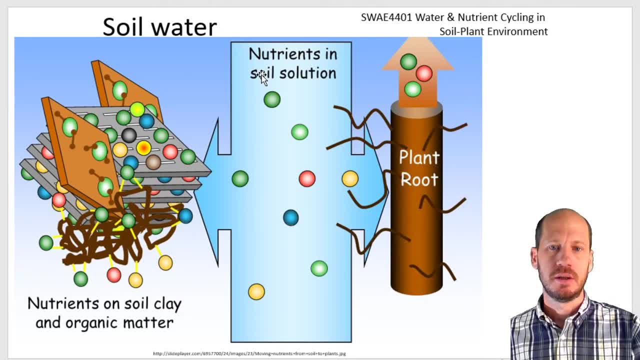 between the soil solid phase, the nutrients in soil solution and their uptake by plant roots. you know the plants will only uptake nutrients. there are soluble ions present on the soil solution, but the soil solid phase acts as storage of nutrients for plants, so as the plants are depleting the solution. 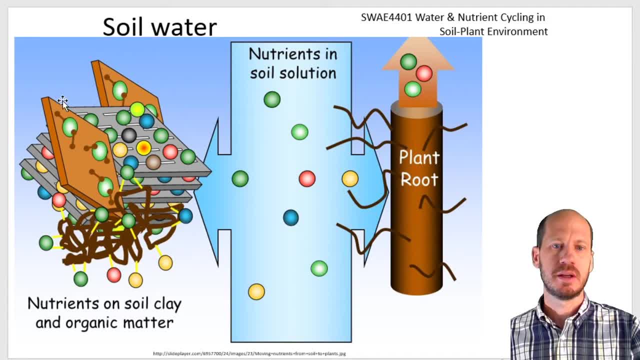 particles, they can consume the nitrogen from the soil also direct the How are the plants going to be bad taking the nutrients from the solution, the solid phase, the solid particles are able to resupply these nutrients to the solution and therefore to the plant. so there is an interface between the roots in the solid phase of the soil, which is 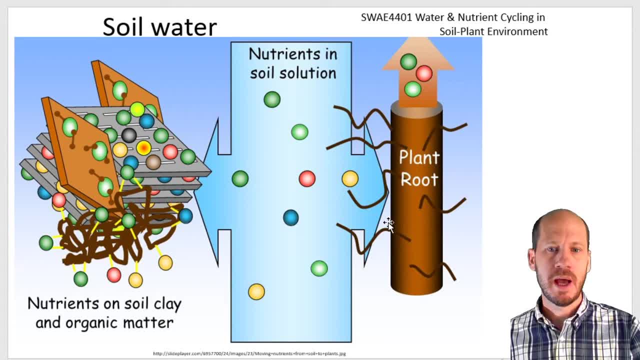 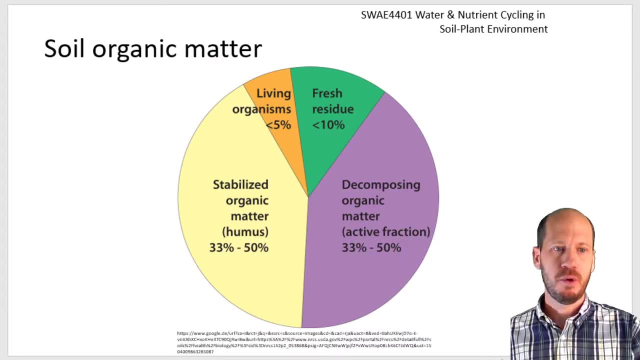 this soil solution when this interplay occurs in a zone of soil call the rhizosphere. yeah, the rhizosphere, alright, so how good does this work? so let's talk. before we move to talk about clays and other types of colloids, we're going to talk. 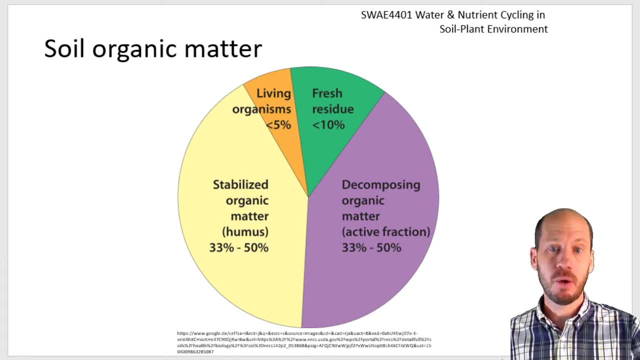 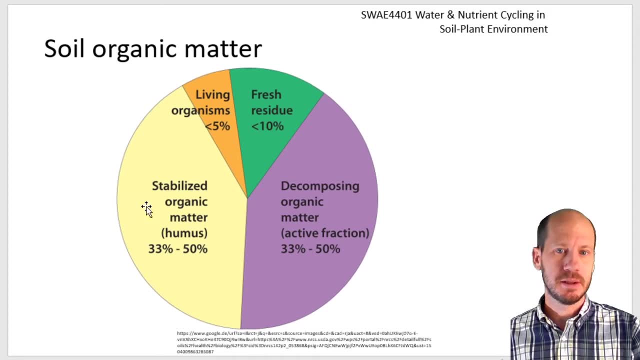 about organic matter. organic matter is very complex and it's strongly conditioning the availability of nutrients to plants. you know, strongly conditioned availability of nutrients to plants. organic matter- we can classify them in different types of organic matter. we have fresh residue, like the, the, the rest of the crops left on the field, the litter. we have living organisms. 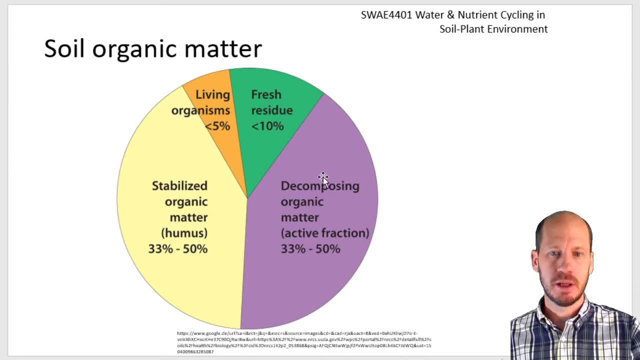 we have decomposing organic matter which is in in some state of decomposition, and you we have stabilized organic matter in soil, also known as humus. some of these humus is stabilized through their interaction with other colloids like clays in the soil or iron- iron- 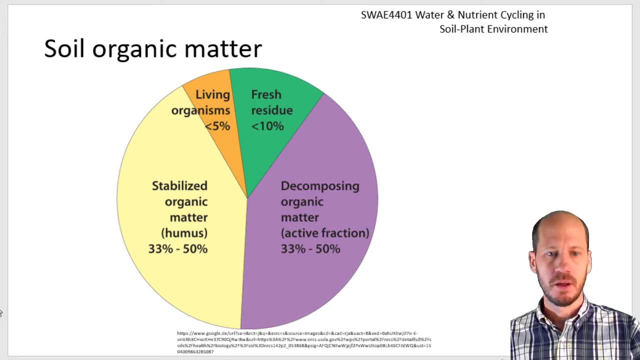 and aluminum oxides in acid solids, for example. but we are interested in two things, and many, many things actually, but in which ways these organic matter are affecting plants, in which ways they're getting. organic matter can help plants in soils, and actually there are three different ways. this 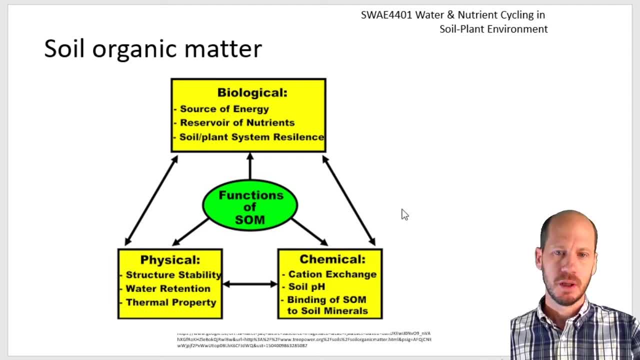 organic matter is helping plants. one is the most obvious one: it's being decomposed and in Ethereum origin, as it is being decomposed, provides nutrients to plants, so in the chemical way. but it's not the only chemical way organic matter is affecting soils. it's also changing the 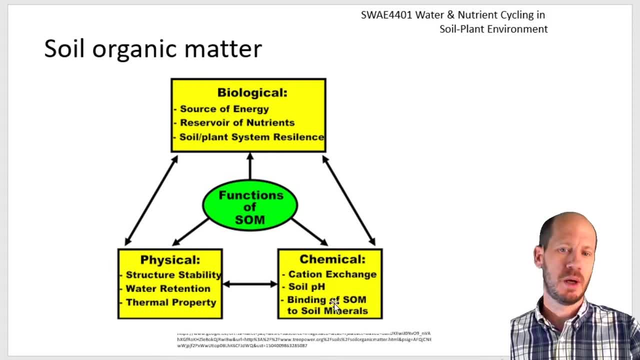 behavior of other colloids in the soil. it's regulating pH is improving the cation exchange capacity- we're going to talk about this concept in a bit- and in physical ways increases the structure of the soil, water retention- and you can use the ricochet �frit6 to increase the structure of the soil in water retention. and石 was very interesting to know we had equal carbon use. 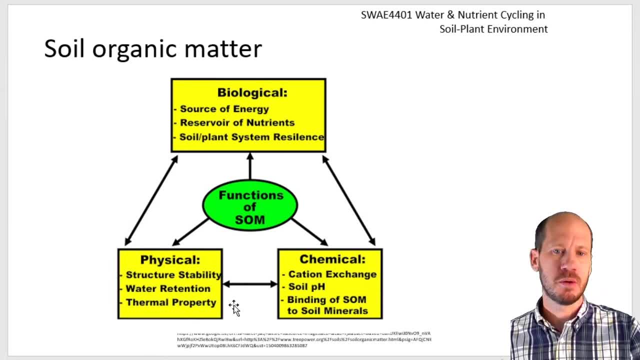 infiltration rates and thermal properties of the soil. But more important also than this, not more important but equally as important- is that organic matter is food for the microbes. it's food for the microbes, The majority of the soil community, the microbial community. they are heterotrophs. 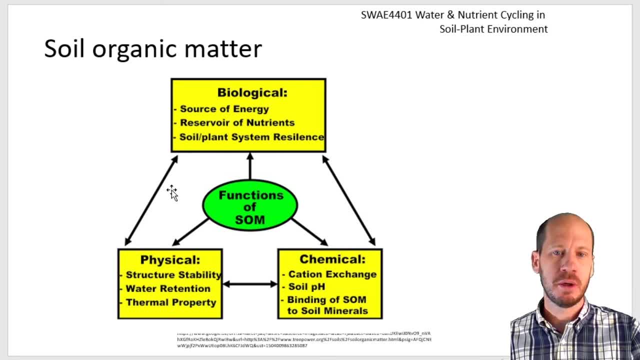 Means. they're using organic matter as a source of carbon, as a source of energy. So these microbes are really important for plant nutrition in many ways: fixing nitrogen, solubilizing phosphors and, in many ways, protecting the plants from pathogens. 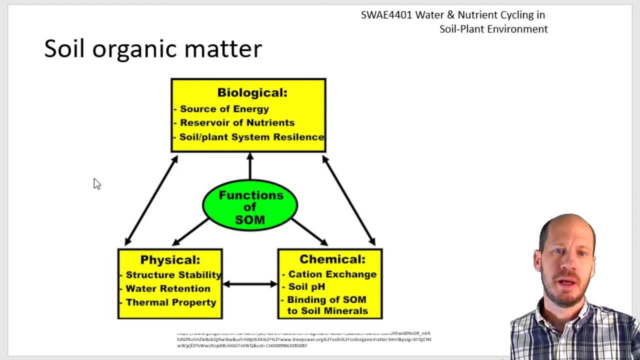 There are many roles of soil microbes in soils And without organic matter, this activity, the activity of the soil microbes, is decreased strongly, yes, strongly. So these are the three, the main ways in which organic matter is playing a role in plant nutrition. 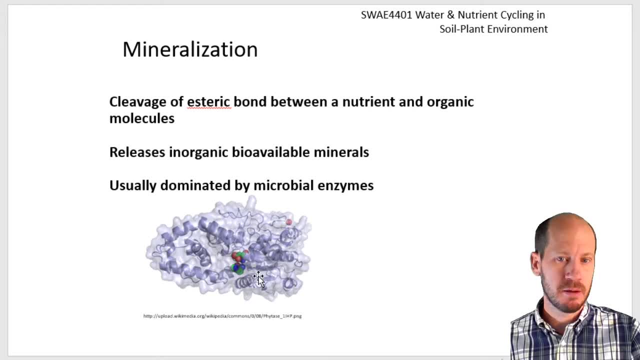 So organic matter can be a source of nutrients by itself by being decomposed by microbes. So how do microbes decompose organic matter? By releasing enzymes into the soil Hydrolysis that break down the bonds between carbon molecules: carbon to carbon, carbon to nitrogen. 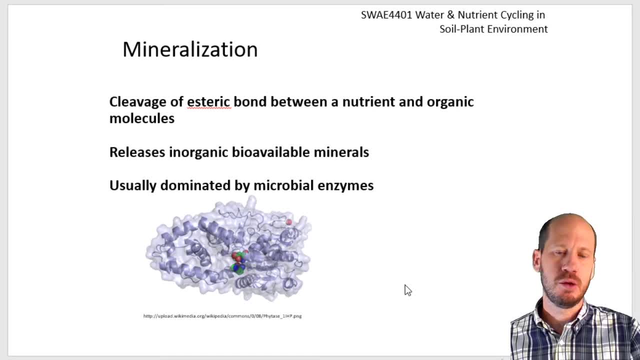 carbon to phosphors, releasing these nutrients into the soil solution and making these nutrients available to plants. So carbon in itself is not from the organic matter, is not a source of carbon for plants, because plants photosynthesize, but it's a source of carbon for microbes. 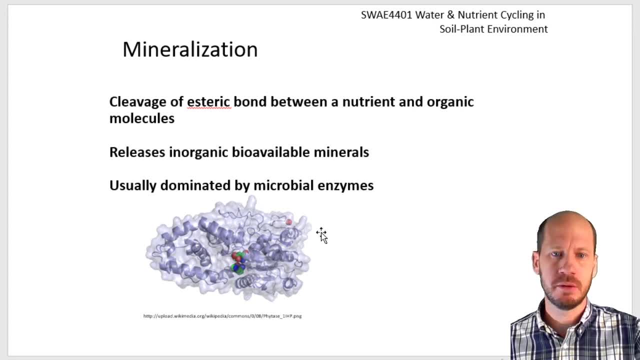 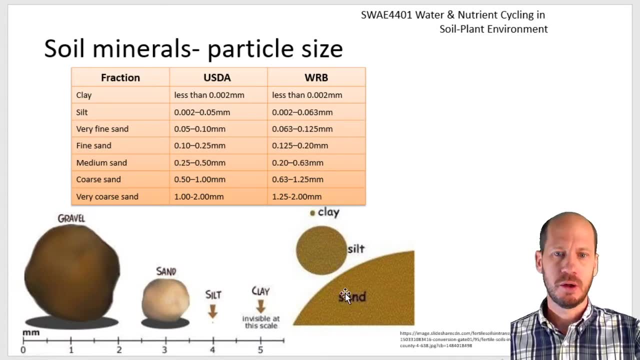 And by doing that it becomes a source of other minerals. And by doing that it becomes a source of other minerals for plants, you know, for plants. Now, talking about the soil particles excluding organic matter, the soil solid phase, we can classify this in clay, silt or sand. 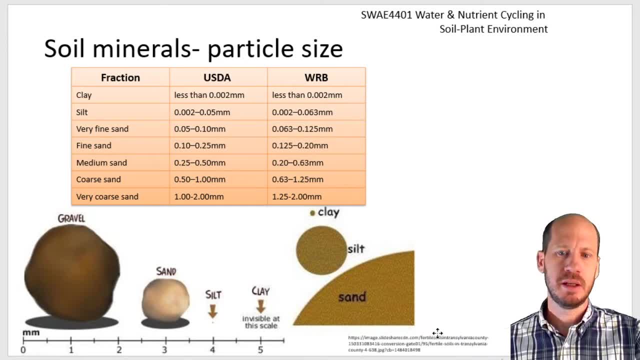 You remember this from introduction to soil and water, And this classification is based on the size. different agencies or countries will have different definition of those sizes, will have different definition of those sizes, Especially when it comes to the silt and clay sizes. 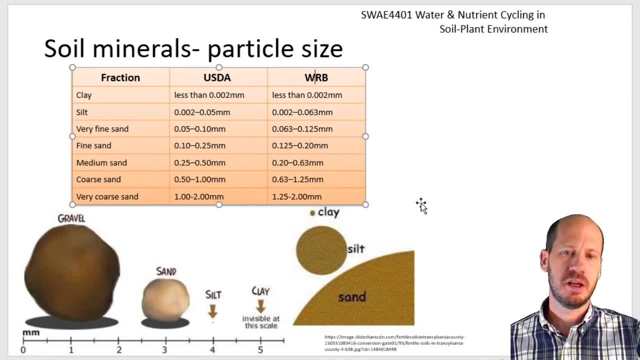 Especially when it comes to the silt and clay sizes. But in general you would say it's just sand. it's a very caress that you can feel it on the touch, The silt. it feels very smooth on the hand, but not sticky. 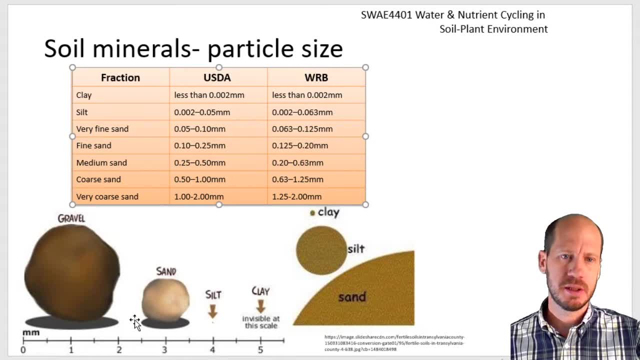 And the clays will be the very sticky substances on the soil. So they're classified by size. but you can also, you know you can- classify them by size, But you can also, you know you can- classify them by size. 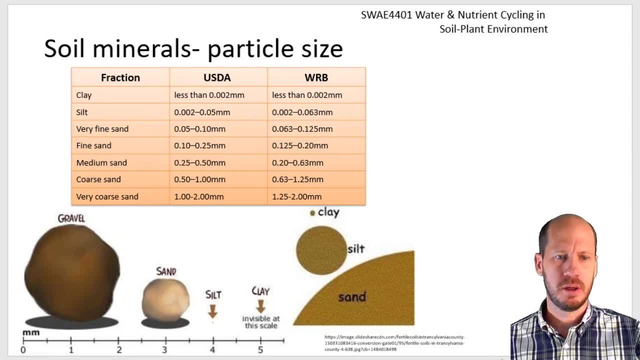 So I classified them by how you feel them in general, Why we are talking about this. we are interested in clays. Yeah, we're very interested in clays. Clays are heavily in conditioning the chemistry of nutrients in soils Because clays- along with uterus, they're colloids. 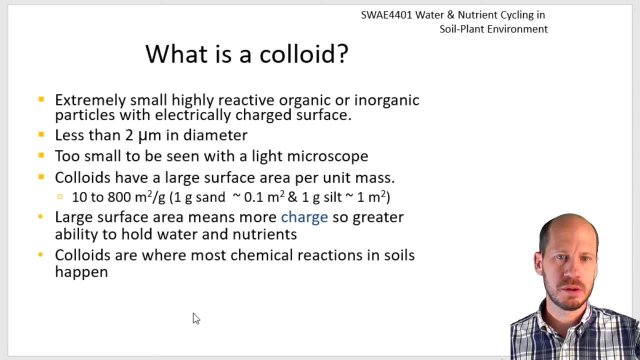 Because clays along with uterus. they're colloids. Yeah, They're colloids. and what are colloids? They're very, extremely small particles. They're very, extremely small particles that cannot be seenVERY small particles that cannot be seen. 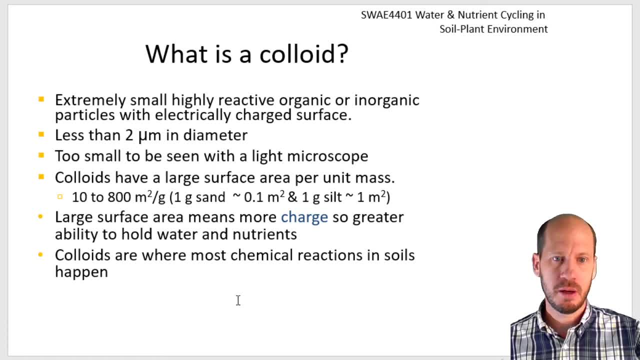 with the light microscope. they need an atomic absorption microscope Because they are small, they have a very high surface area and they have charge. The main thing about these colloids is they carry charge And this charge needs to be compensated in the soil solution by ions. 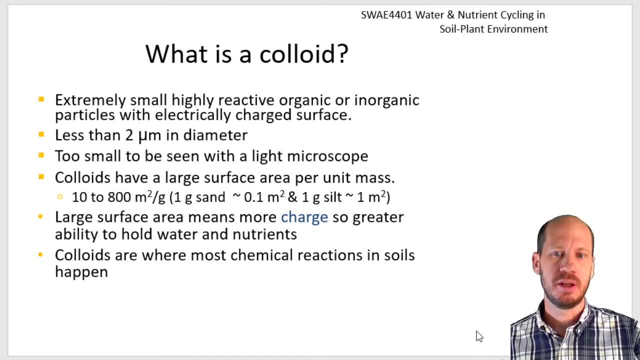 And therefore the ions that stick to these colloids. they are adsorbed into the colloids And this soil. because of the charge of the colloids it acts as a reservoir of nutrients. If you have charge on the solid phase, you need to compensate that charge with ions And those ions 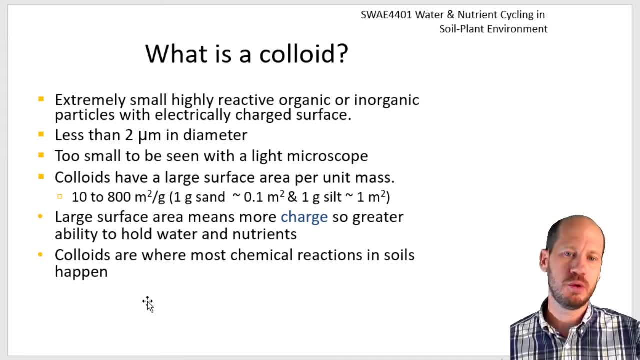 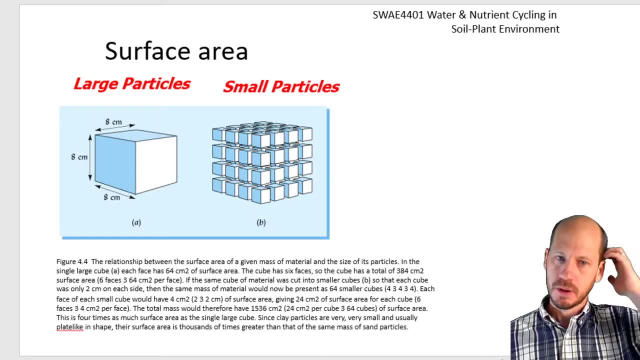 are the nutrients for plants. The nutrients of plants are ions that can be stored, adsorbed on the solid phase. This is just explaining really quick, reminding you the consequences of surface area and that large particles will have less surface area than small particles. 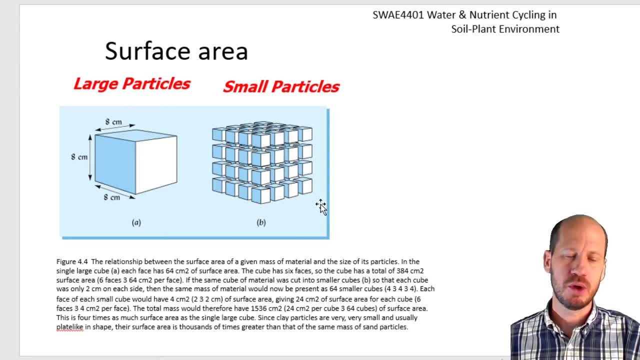 Because if you think about how you split them, they will show more faces of these particles and therefore they will have more exposed area. So the reaction between the solid phase and the solution phase and the soil water, the nutrients are interchanged between the solid phase and the 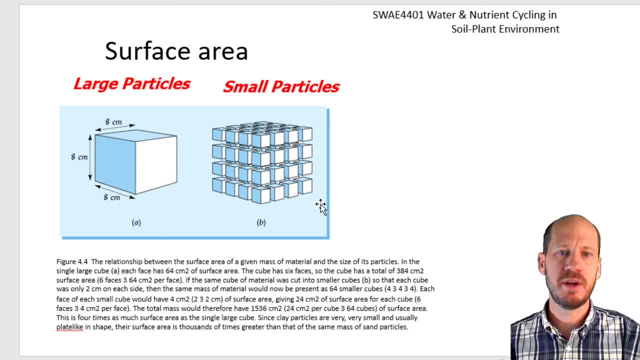 solution through those surfaces. The more surface area that you have, the more reaction you will have, the more the capacity of the soils of storing nutrients. The amount of surface area is directly proportional to the capacity of the soils of providing nutrients for plants. 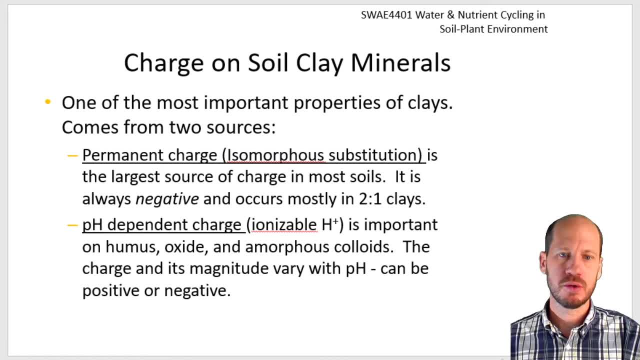 And the charges that you have on them. on the clay particles. they are divided in two different types of charges: permanent charge and the other one is pH dependent charge. The permanent charge does not change when you change the pH of the soil solution. If you change the. 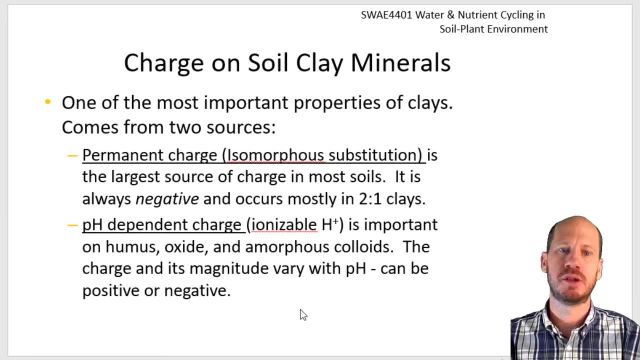 pH of the soil solution. there's no change on the permanent charge. The reason for that is that the permanent charge is originated inside the structure of the clay by a process that is called isomorphous substitution. The process called isomorphous substitution. 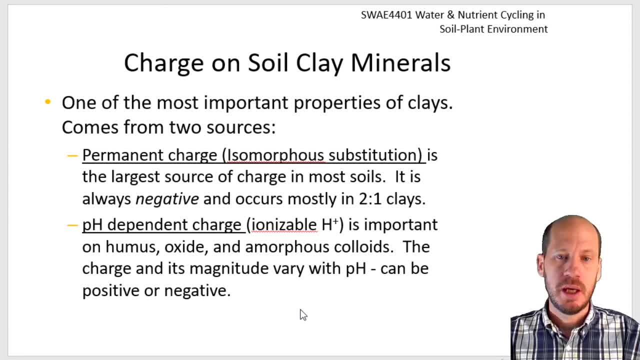 Where is the pH dependent charge? It's a charge that is generated on the surface of the clay. Therefore, you can protonate and deprotonate those oxygens on the surface of the structure. By doing that, you can change the amount of. 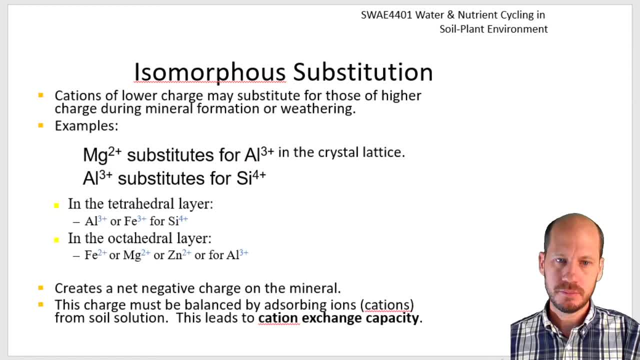 of charge that you have. We'll explain that in a bit. The isomorphous substitution: when you, in the original structure from the clay, you have some ion of higher valence and this ion of uh, like aluminum, for example, or silica, silica can be substituted by by. 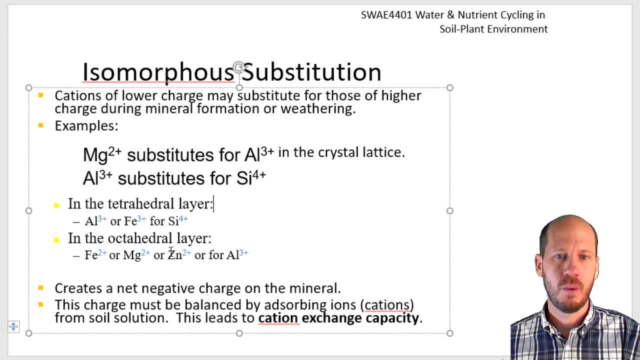 aluminum and therefore you lack. yeah uh, one one, uh, um one charge and it becomes negatively charged. so yes, the isomorphous substitution is originated inside the structure and therefore cannot be compensated by covalent bonds to the structure. so the covalent bonds would make a stable bound. 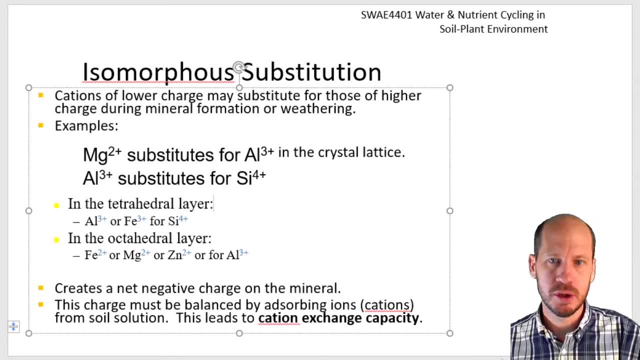 whereas if you have the, the isomorphous substitution, it can only interact with ions by electrostatic interaction, not by covalent bonds, and therefore these ions can easily solve, absorb and dissolve from the solid phase. so just a clarification: adsorption in is when it sticks to the solid phase. 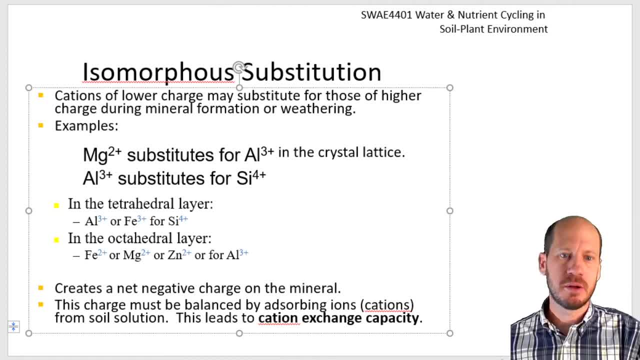 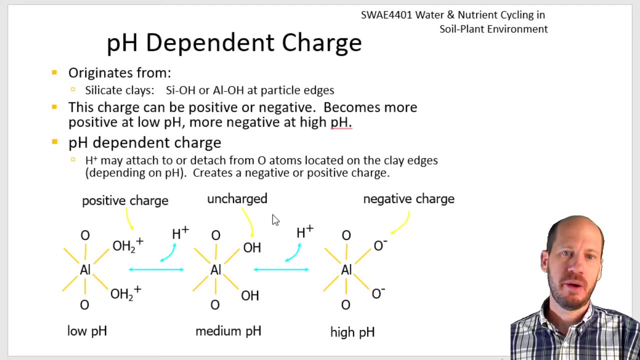 desorption is when it's released from the solid phase. yeah, so this isomorphous substitution is generating permanent charge on the soil, the charges that that are independent of ph, whereas the ph dependent charges. they form on the surface of this glaze and on the on the clays. they're more present on the, the edges, in organic matter, all over the organic. 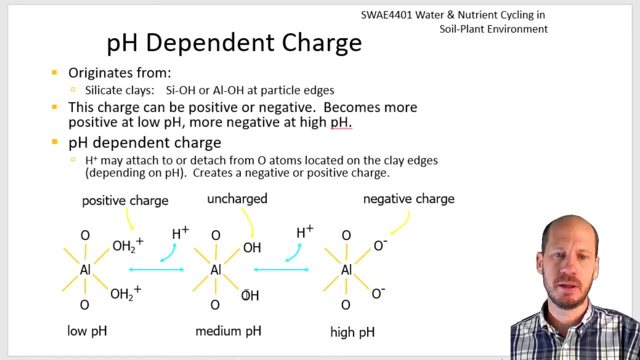 matter in the iron and aluminum sides all over them, but on the clays, on the edges of the lattices of of the clays. how it works for the ph dependent charge is when you have low ph you have a high concentration of protons on the solution. those protons will 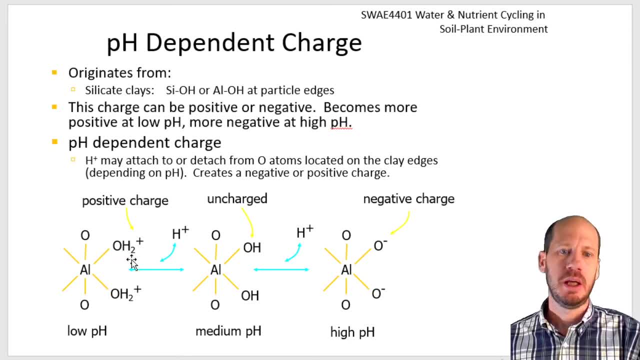 will stick to the, the hydroxyl, and by, by protonating the structure, you can you create a positive charge. if you start rising the ph, you reach a point where it's these protons are released back into the solution, and this point is called the isoelectric point. 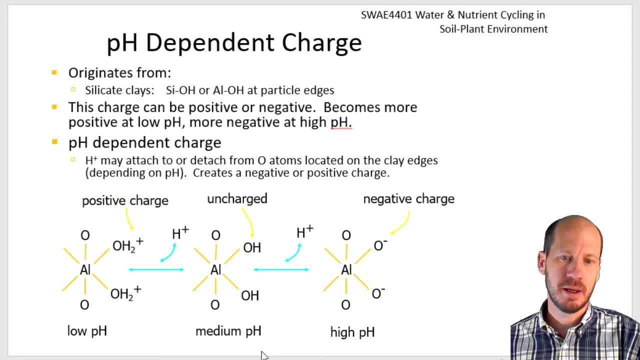 or the zero point charge of the clay. yeah, if it's a a ph dependent charge, clay, clay, you will have that at some point. you have a net charge is zero. The net charge zero is the isoelectric point or the zero point charge of this clay. If 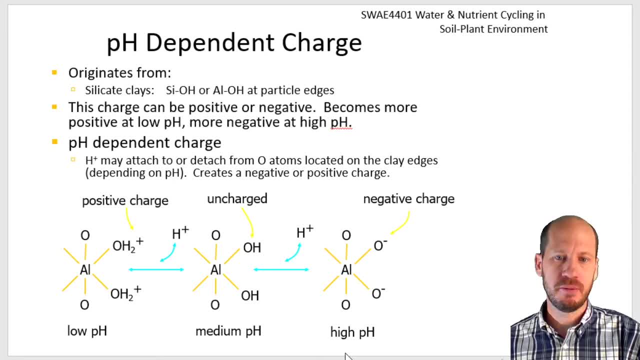 you continue increasing this pH, the concentration of hydrogen and solution becomes so low that even it will lose those protons and generate negative charge. So normally the zero point charge is on the acid range. so most of the soils will have negative charge as pH dependent. but how much, how many? 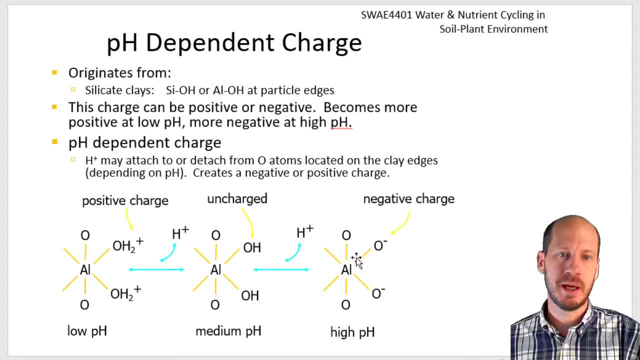 negative charges. the amount of negative charge by pH dependent charge is regulated by the pH of the solution. So the more you increase the pH you increase also the amount of negative charge as pH dependent. So this is only review from introduction to soil and soil. 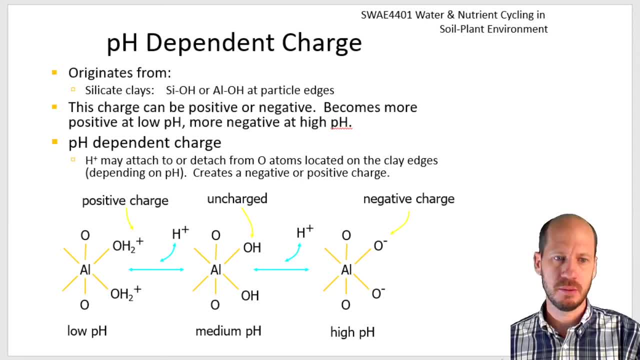 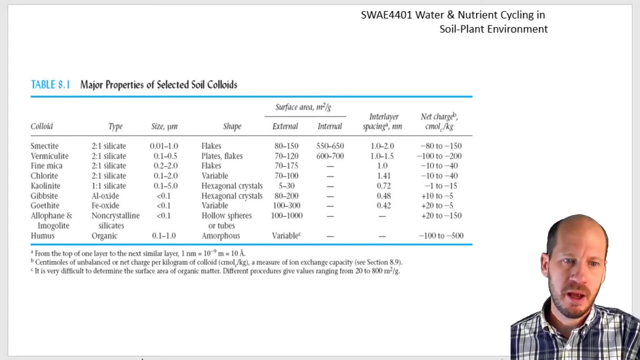 chemistry. These concepts are already given before, but it's worth reminding why we care about this in the context of plant nutrition. It's about the nutrient interchange between the surface of this clay and the solution and with the plants. And here it goes. yeah, the, the, the. this different clays will have different properties, different 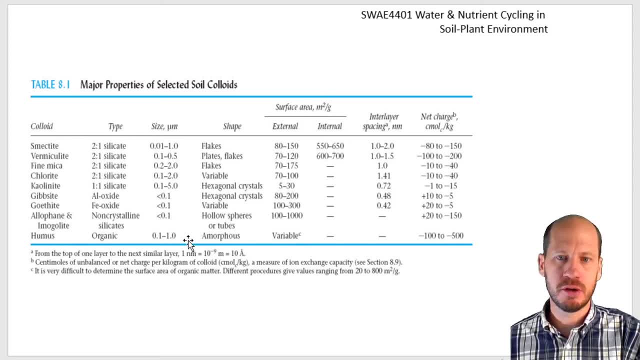 clays will have, including the humus. they will have different amount of charge and you will have different types of charge. yeah, a different surface area. so all this we condition how much ions you can absorb. so the the the highest amount of charge per gram of material is on humus, and after that you have the two to one. 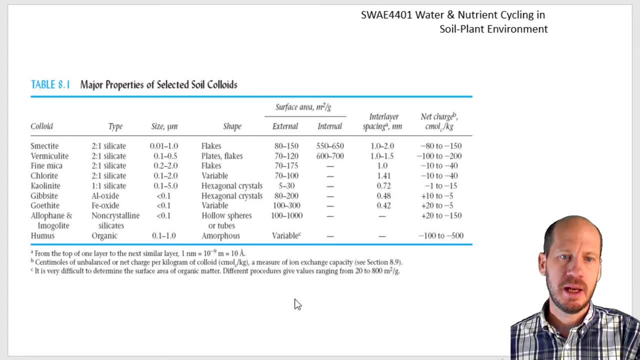 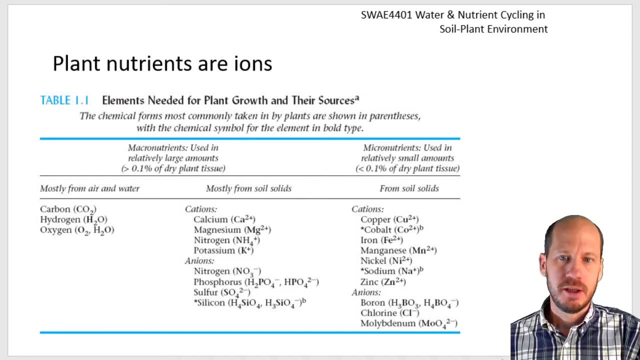 clays being a more charged, and then after that you have the one-to-one clays And, of course, the nutrients that plants use. they are ions. They are ionic nutrients, either cations or anions, but these ions interact with solid phases. If they are positively charged they will be attracted to. 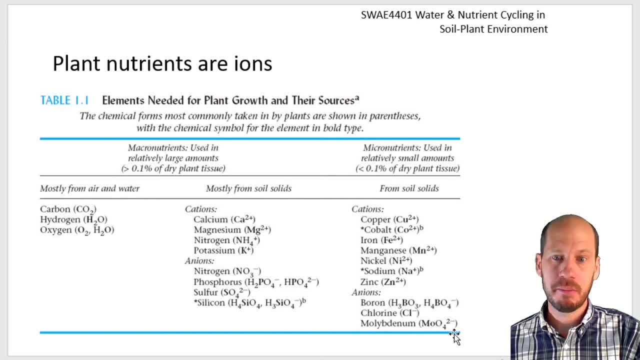 the surfaces and if they are negatively charged, they can be bridged into these surfaces by another cation. So if you have, for example, calcium, calcium can interact with the phosphate and with the surface of a clay, at the same time bridging those anions. 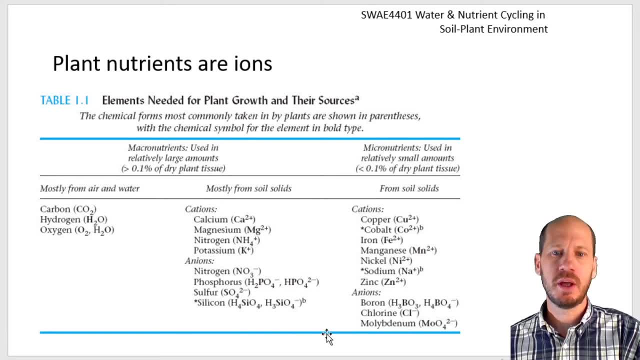 so they can absorb to the solid phase. So both cations and anions will interact with the solid phase. Some ions will interact more strongly than others And these will regulate also their behavior in soil. How mobile are they in soil depends on how strong the interaction is. 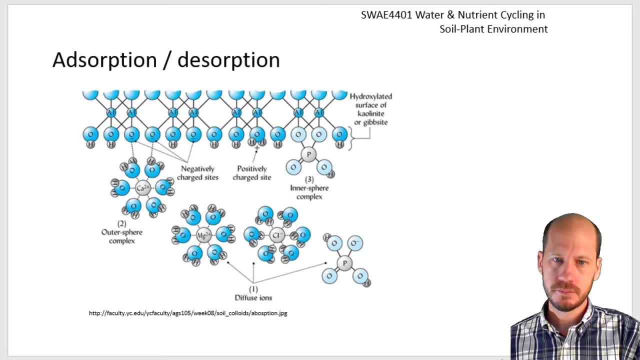 between these ions and the solid phase. So here is an exemplification of the adsorption process. and then you have a phosphate molecule which is forming here inter-sphere complex adsorption. The inter-sphere complex is when it binds valently to the surface of this colloid. and here this phosphate here is diffused or not. 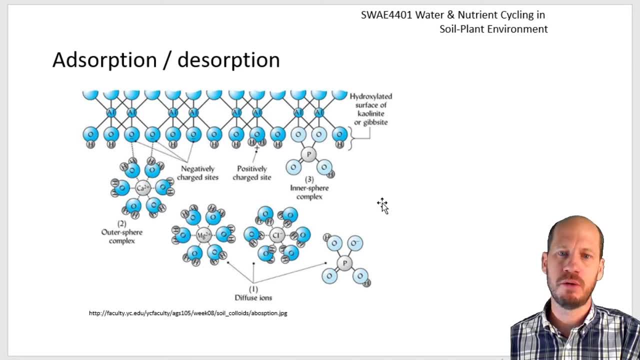 not absorbed at all, but you can form hydrogen bonds and we have an electrostatic interaction between different ions, hydrated ions, and the surfaces of these clays or colloids in the soil, the. the strength and the behavior of this interaction between the solid phase is measured by the absorption isotherms. yeah, absorption isotherms. here are some examples. 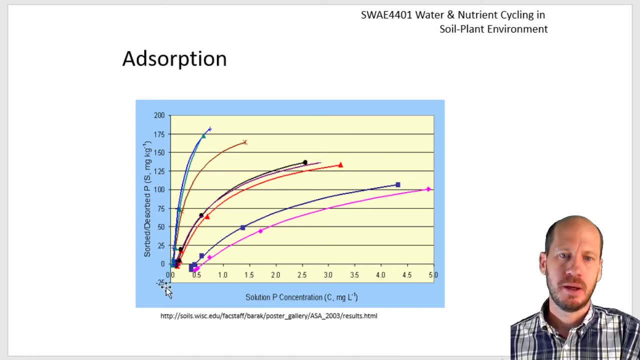 of absorption isotherms. on the y-axis you will have the amount of adsorbent ion and in the x-axis you will have the amount of the ion on the solution. the more ion on the solution, the more you will have on the solid phase. But it reaches a point. 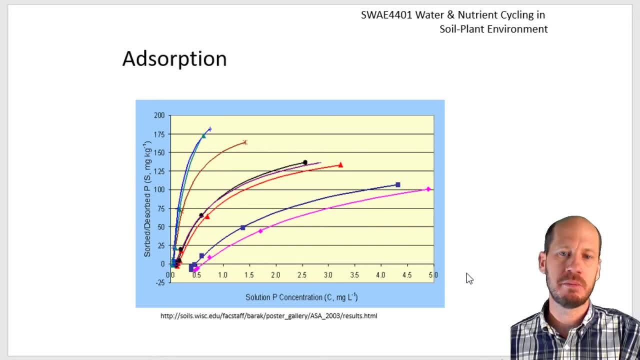 that the solution concentration is so high that the solid phase becomes saturated, So this becomes flat. The closer this curve is to the y-axis, the higher the affinity of the ion for the solid phase. The lower this curve is, the closer it is for the x-axis. 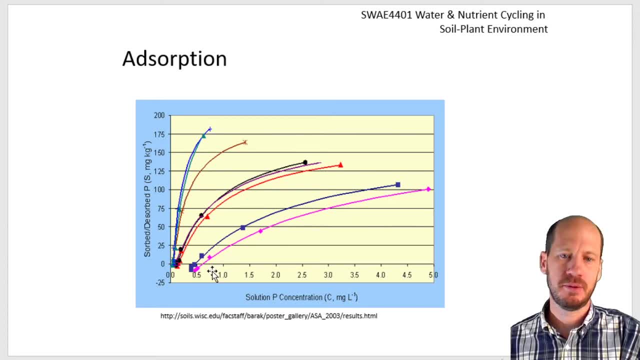 the lower the affinity for the solid phase. So we are talking about how strongly, with how much energy, an ion interacts with the colloid in the soil. So we have the colloids regulating how much charge you have. but the ions also compete with themselves with each. 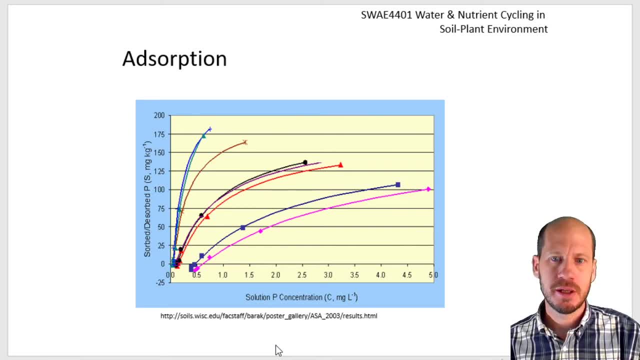 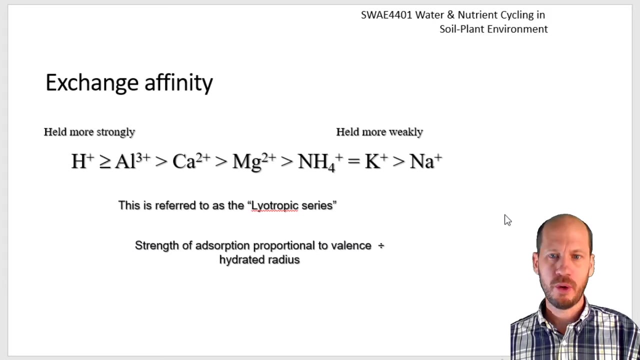 other. for these adsorption sites on the soil. They have competitive adsorption. Some are more attracted to the colloids than other ions And if we compare how attracted these ions are to the solid phase, we can form an order of energy in which these ions are interacting with the 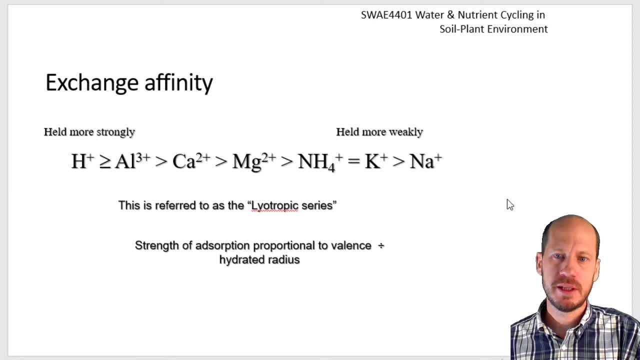 solid phase, And the order of this energy of interaction is called the lyotropic series. The lyotropic series organizes these cations in order of strength of interaction with the solid phase. So hydrogen is the one with highest affinity for clays and iron oxides, aluminum oxides and organic 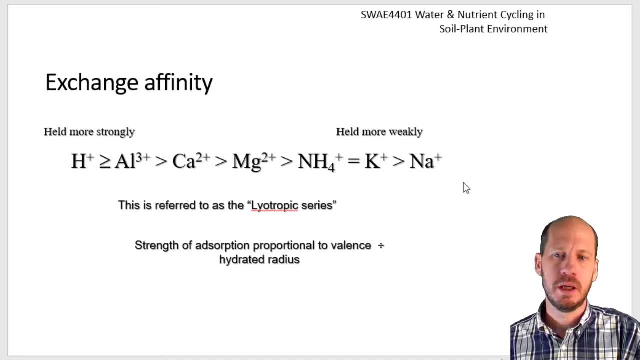 matter, whereas sodium is the one that has lower affinity. So you will find sodium and potassium most likely in solution, whereas you will find calcium, aluminum and hydrogen most likely associated with the solid phase. So they are less mobile if they have higher 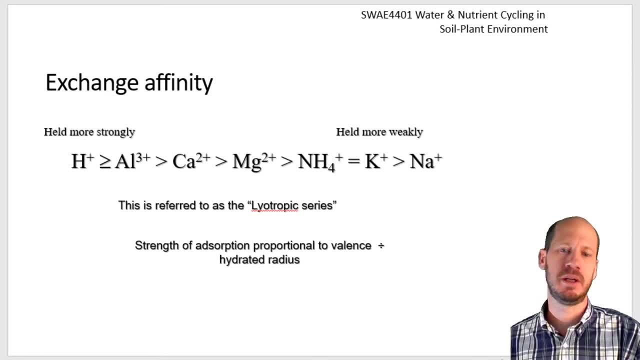 affinity. They are more mobile if they have lower affinity And if you have more. this is adsorption is a function of both this affinity, but also the concentration. If you have too much of an ion, even if it has low affinity, it will be able to displace other. 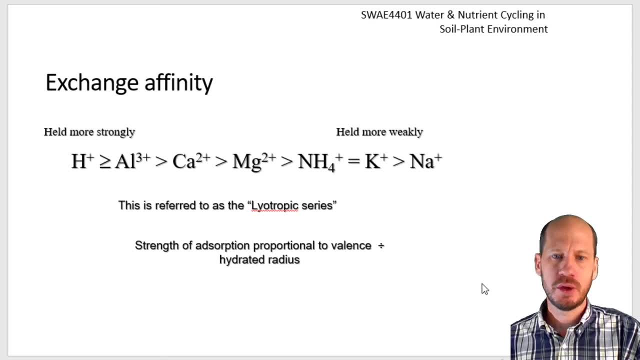 ions from the solid phase. So these two things are important In adsorption. one is the affinity exchange, affinity- and the other one is the concentration of these ions. Why now? Why one ion will have more affinity than another one? The reason is what we call. 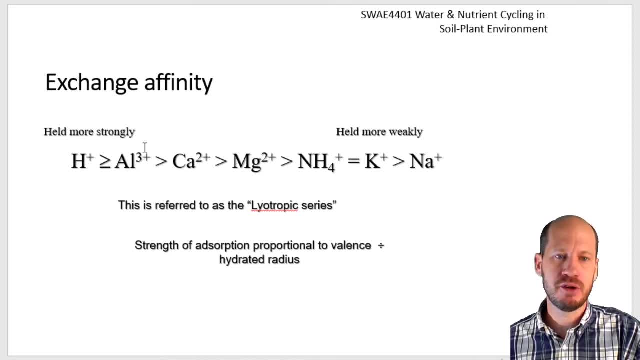 the charge density. If you imagine a hydrogen has only one valence, one plus, but is very, very small In the, in the same position, when you have one sodium, you can fit many may hydrogen. So in the same space the density of the charge will be very high. So that's. 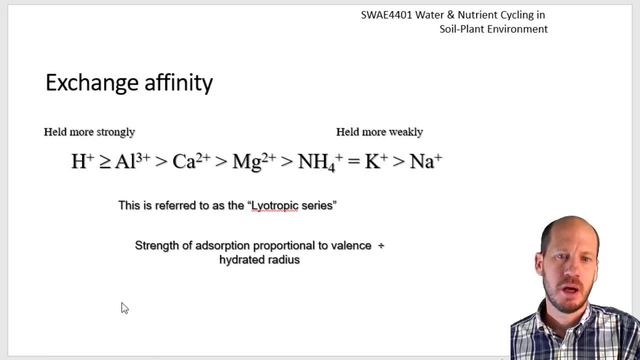 the charge density of these ions. Also, it's what regulates this exchange affinity. The smaller they are for the same valence, the highest affinity. The bigger they are for the same valence, the higher the affinity. the larger is the affinity in those valence smelling. 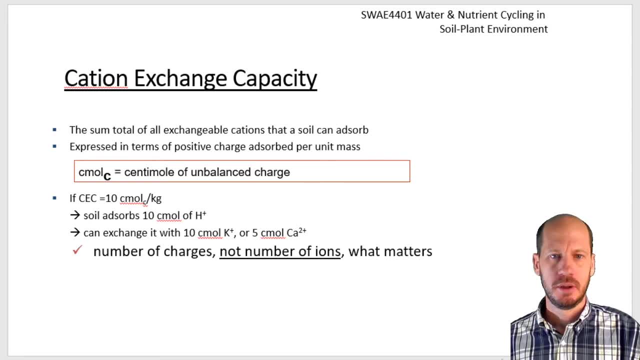 theirve going to statistical velocity have for participants. So I will be pointing you exactly to battery fading and normalization of intuition, detailed. So why second that? Libert maze is to measure weight and time and temperature. лучше than linear smartness, the lower the affinity. So we come to this concept that the solid phase of the 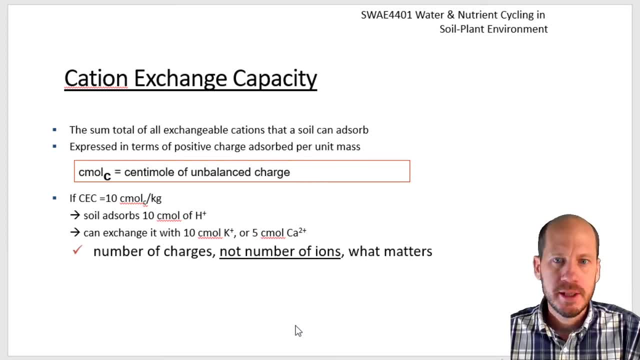 soil, the soil by itself, all the colloids add together. if you sum up all the charge that the soil possess, all the charges together of the soil, they account for the cation exchange capacity. The cation exchange capacity is the number of charges. It's equivalent to how much charge you have on the 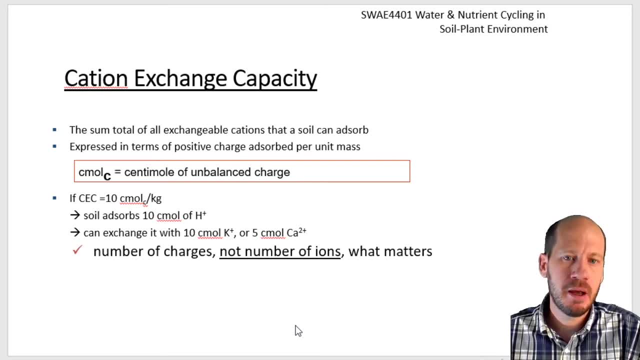 soil. You measure them by adding up the ions, but it's not a sum of the ions, it's the amount of the charge that the soil possess. This is a measurement of the capacity of the soil to retain nutrients. The highest, the cation. 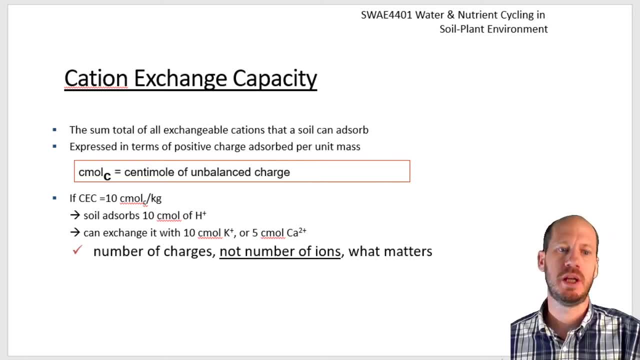 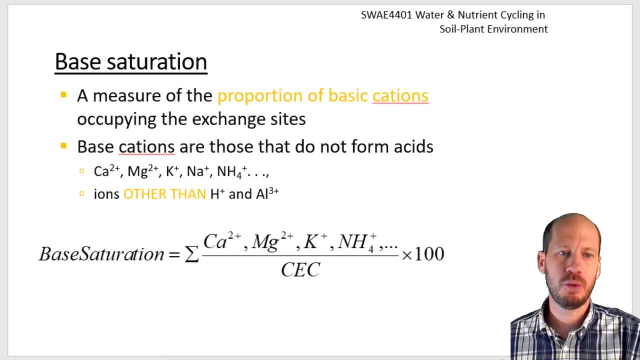 exchange capacity, the highest, the capacity to retain nutrients. You can have some calculations about cation exchange capacity, but we will not worry about that at the moment. The next concept is base saturation. You have two types of ions on the soil: You have bases and you have acid cations. You have hydrogen and 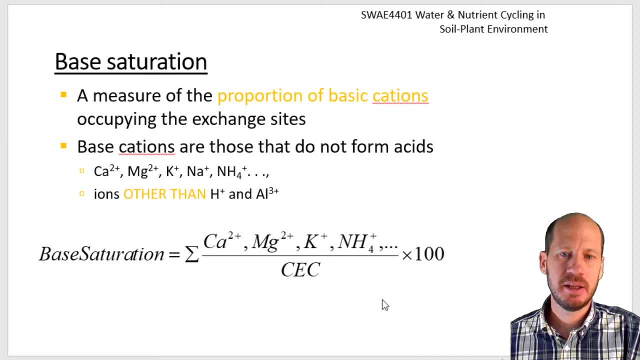 aluminium and iron. They are acid cations, whereas all the other cations they are bases. Why do we classify like that as bases or acid cations? It's because of the reactions they had When they leave the solid phase. do they increase the pH or 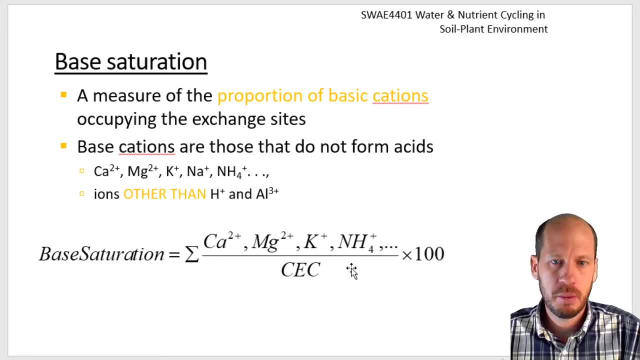 do? they decrease the pH, And this is the concept that we have. If they increase the pH, we call them bases. If they decrease the pH, we call them acid cations. Okay, So if you release a proton, by itself it's already decreasing the pH, okay. 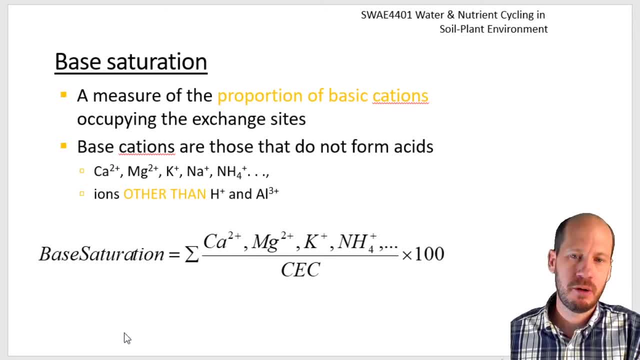 And aluminum also, because the aluminum forms hydroxides and iron also forms hydroxides on the soil, it will also cause the same effect. yeah, If you release that into solution, you will take some hydroxyls and by taking some hydroxyls you will increase the concentration of H+. 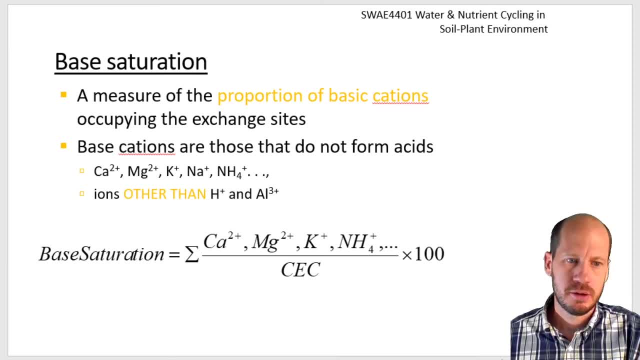 But that is for another lecture. yeah, pH by itself it's very important for plant nutrition. yeah, Base saturation is how much of this cation exchange capacity is occupied by bases? yeah, But the bases and the protons, the protons in the system, they have an effect by itself on plant nutrition. yeah, 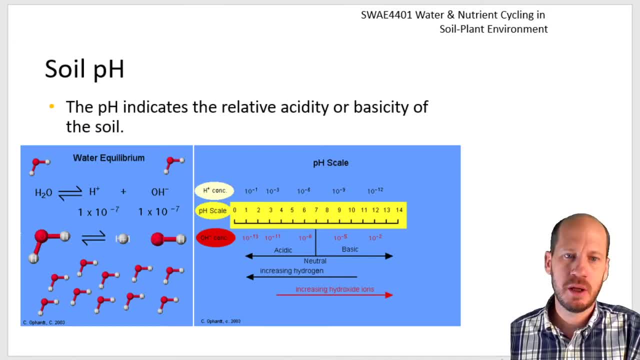 So pH? what is pH? Just reminding you again, pH is the concentration of H+ in any solution. yeah, pH is the concentration of hydrogen. And why do we care about pH? Because the water by itself dissociates H+ and OH. 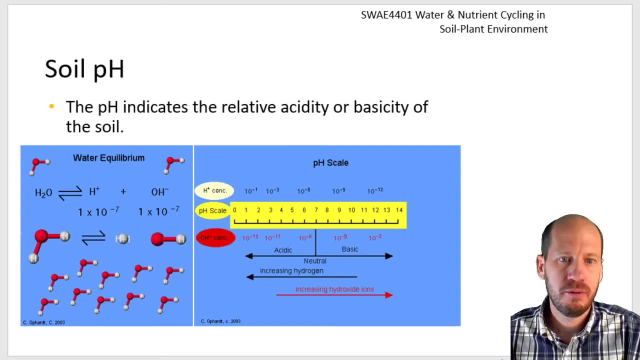 So pure water will have a concentration of 1 times 10 to the minus 7 hydrogen free on the solution, free on the water. Pure water at pH 7, neutral conditions, will have a concentration of 10 to the minus 7 moles per liter of hydrogen. 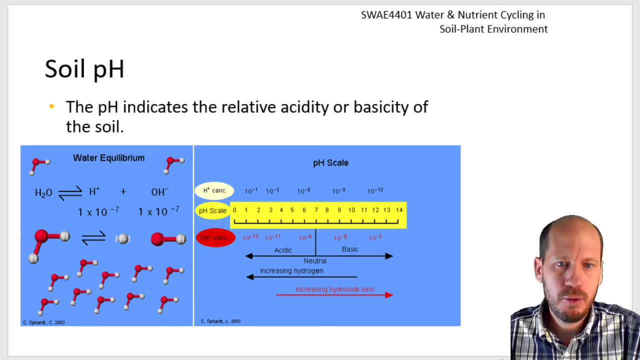 So this is neutral condition. If you increase the amount of protons, you increase, You decrease the pH. If you decrease the concentration of protons, then you increase the pH. So it's a log scale, It's an inverse log scale, yeah. 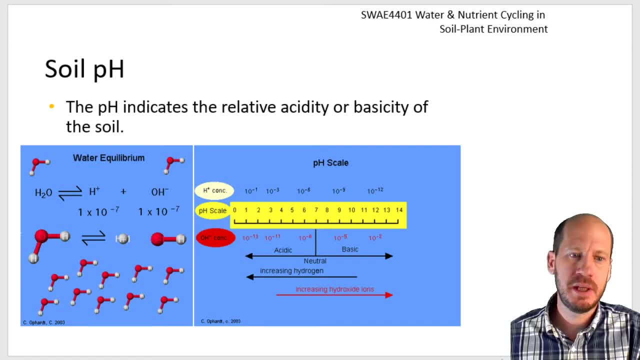 How does it work? the inverse log scale? It means that if you change one point pH, you increase 10 times the concentration of hydrogen Between 7 and 6, there is 10 times more hydrogen at 6 than there is at pH 7.. 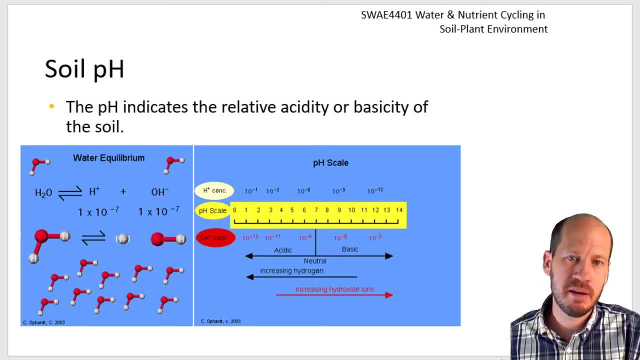 And if between 7 and 8, there is 10 times more at 7 than there is at 8.. So it's always working. It's a negative of the logarithm of the concentration of hydrogen, So it works in the inverse manner. 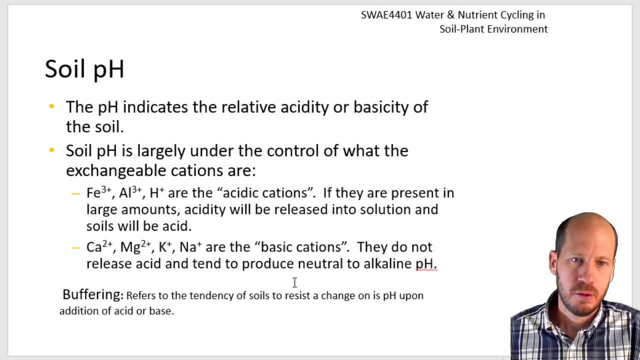 So pH controls a lot of things in soil. We already seen that pH is controlling the pH dependent charges. So pH controls a lot of things in soil. We already seen that pH is controlling the pH dependent charges. Some charges of the soil are increasing or decreasing. 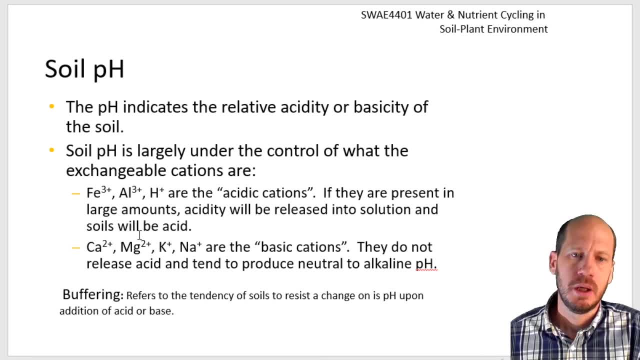 based on the pH of the soil solution, But it's highly regulating the experience of the plant, of the soil The plants will have to deal with. The acidity of the soil can hurt the plant through the release of toxic ions like aluminium, for example. 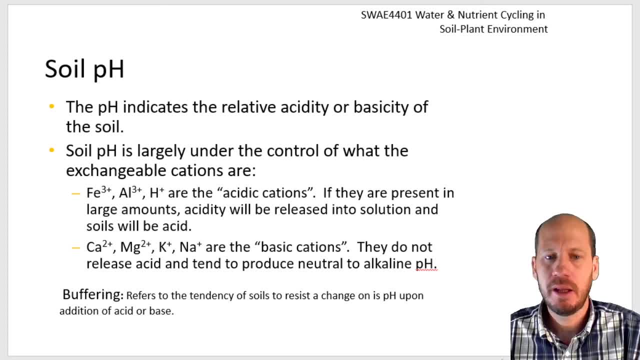 Aluminium will be very toxic to plant roots And it only occurs when you have very acid pH. So when you have very acid pH, you will need to regulate this pH up, And when you have very alkaline pH, you need to regulate that pH down. 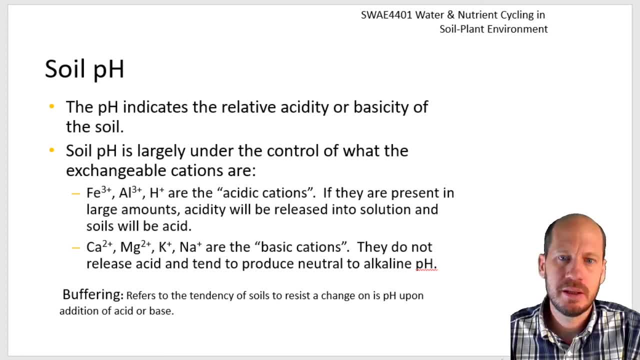 And the main reason for this is that the solubility of ions on the soil will be regulated by this pH. The ions can precipitate. The ions can precipitate or be soluble, And this solubility, it's a pH-dependent solubility. 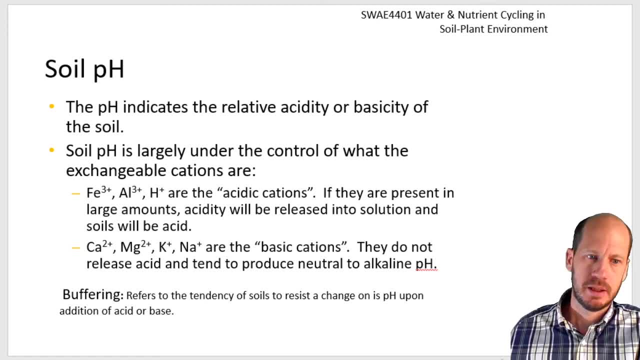 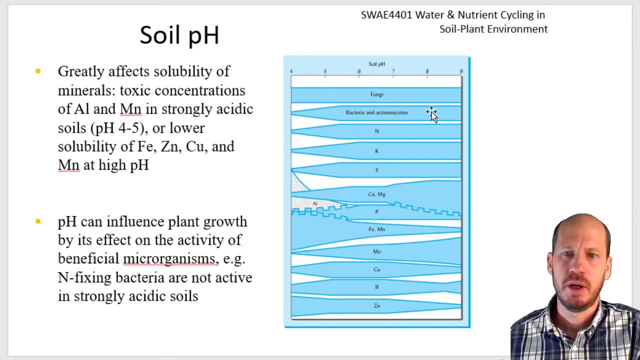 And this solubility. it's a pH-dependent solubility. Let me try to show here- This is the figure explaining this solubility of different ions in soil solution at varying pH And you will see that near neutral condition at acidic condition. 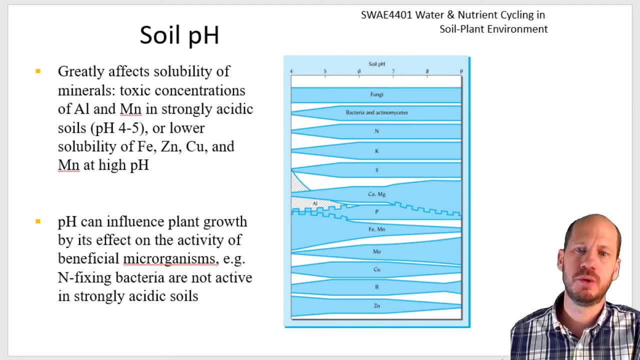 is where we have that most nutrients are soluble. So this is the best range of pHs for plants. So this is the best range of pHs for plants. So this is the best range of pHs for plants. We should always search that the soil pH will be somewhat near acidic neutral conditions. 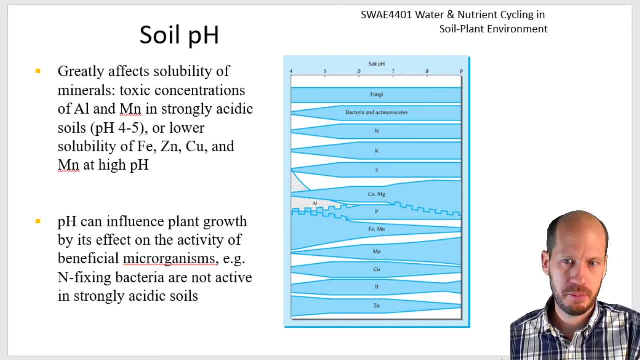 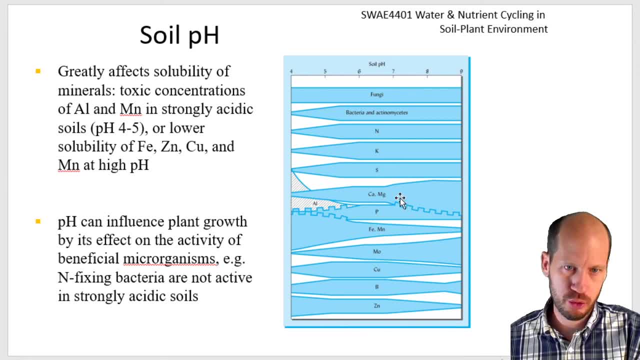 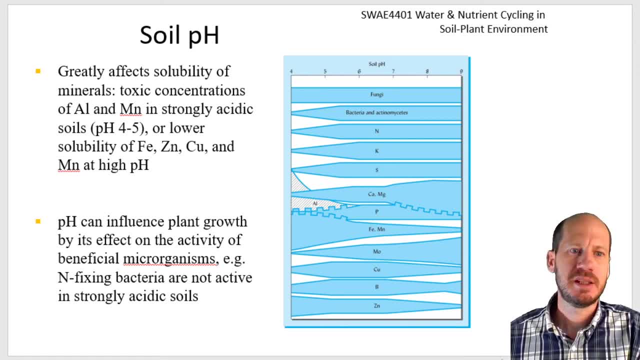 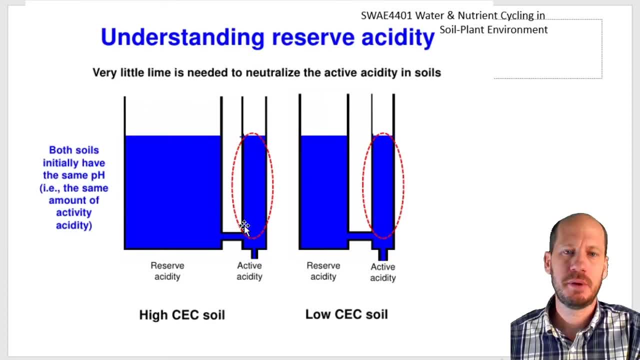 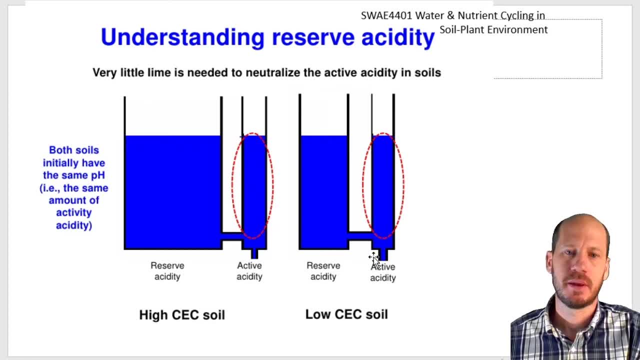 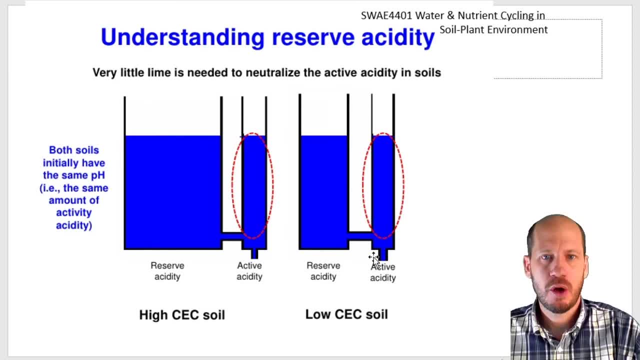 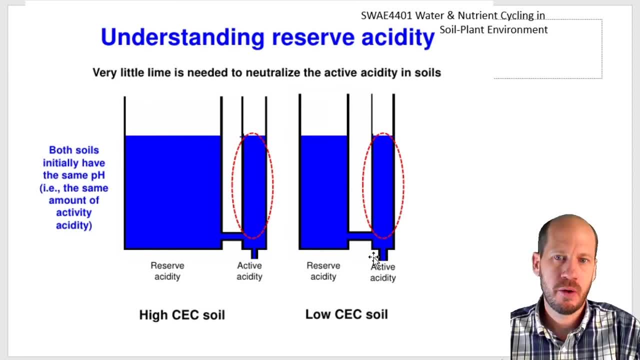 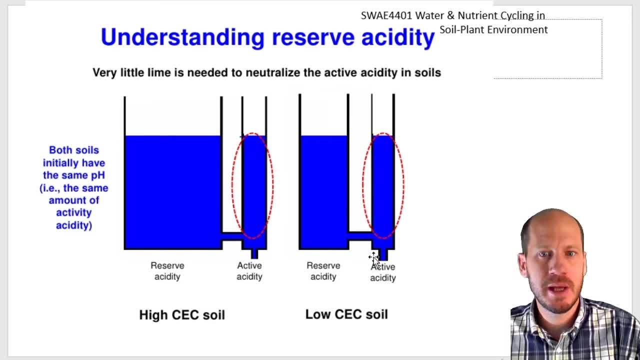 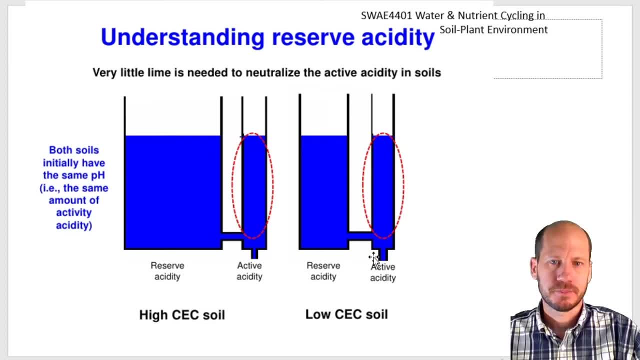 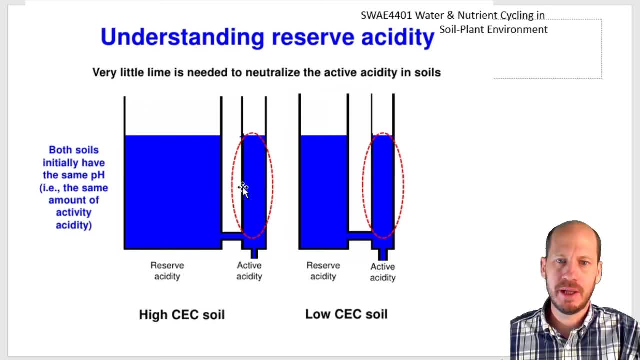 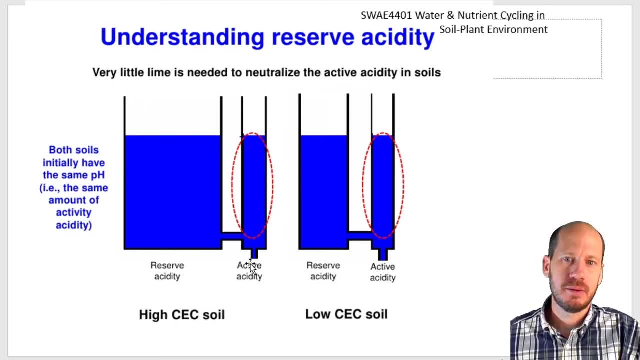 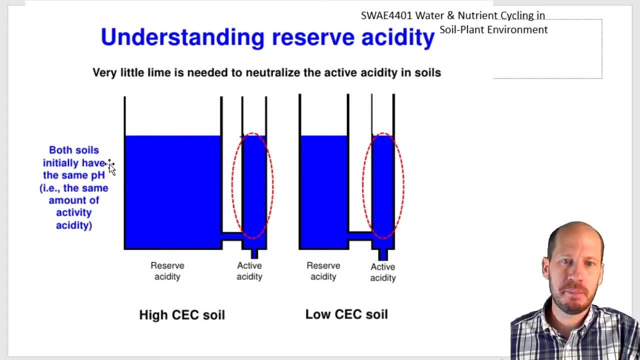 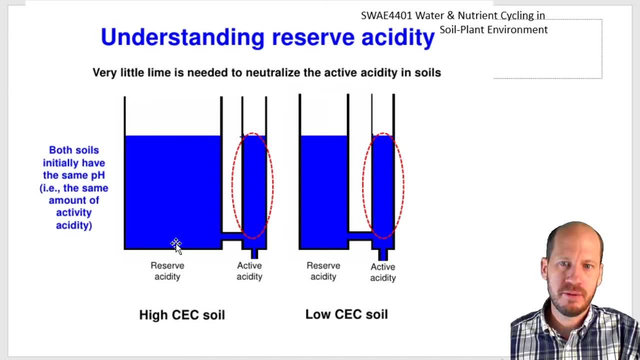 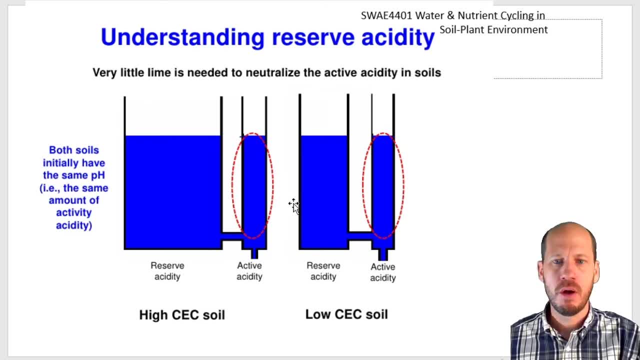 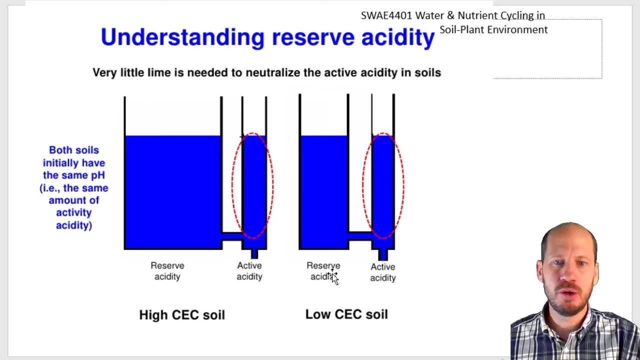 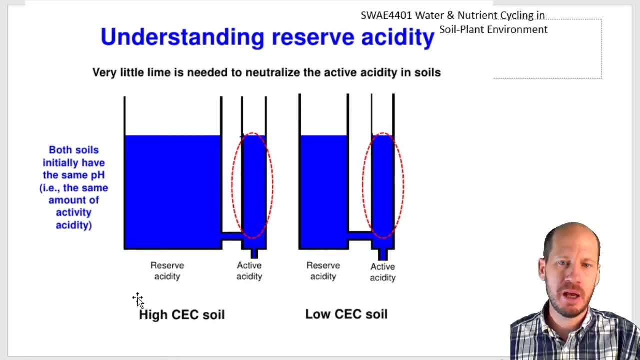 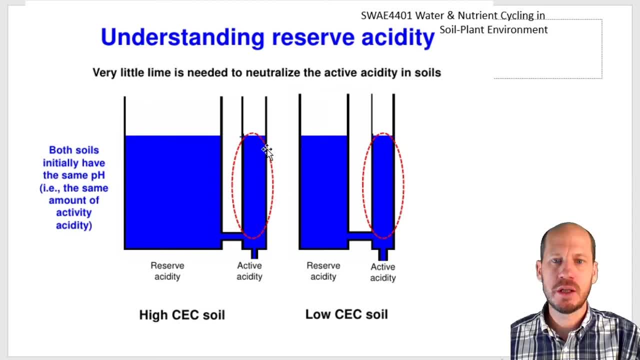 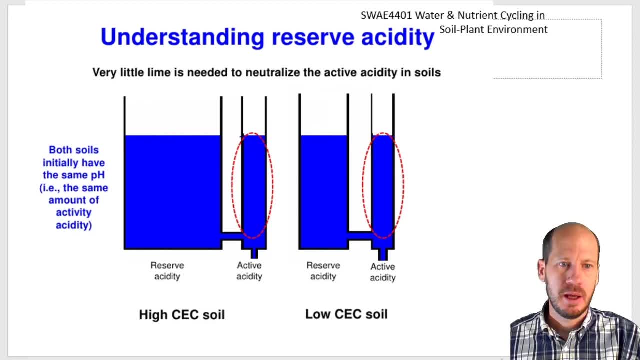 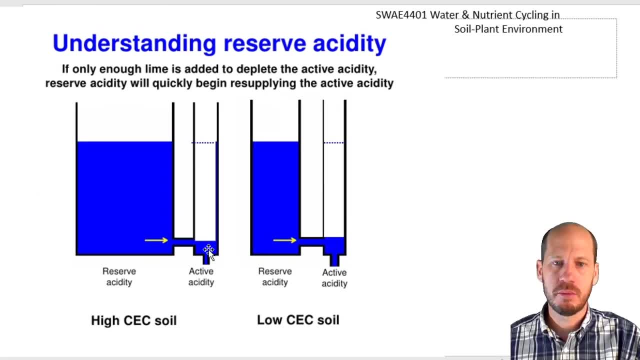 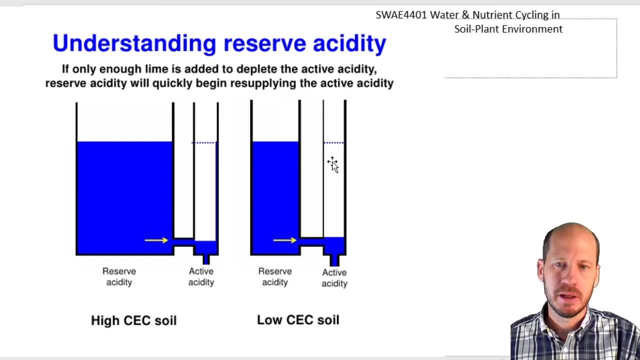 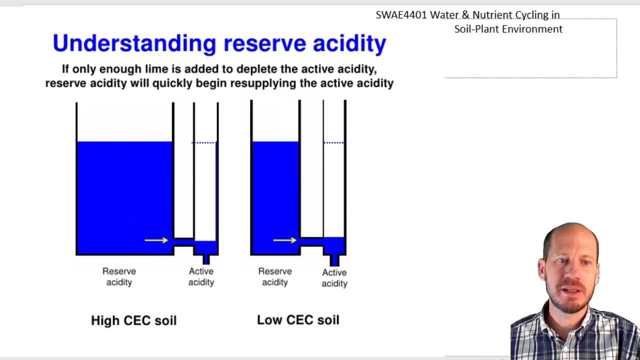 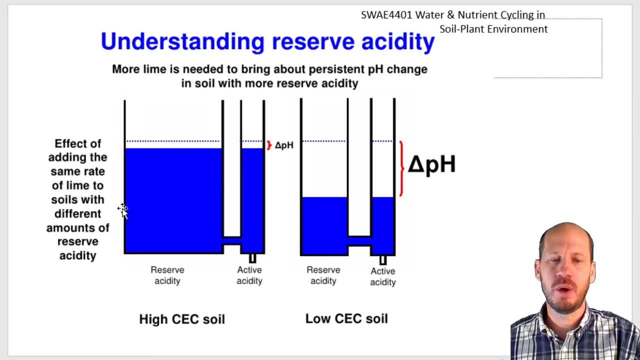 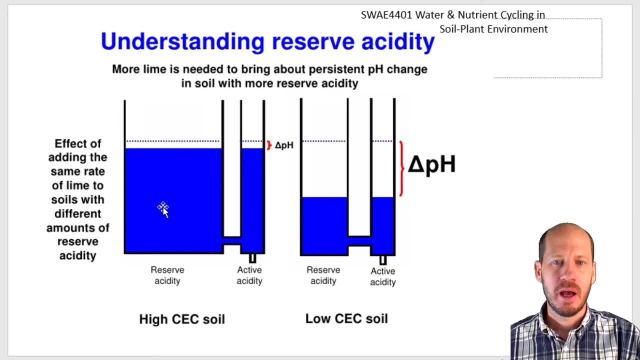 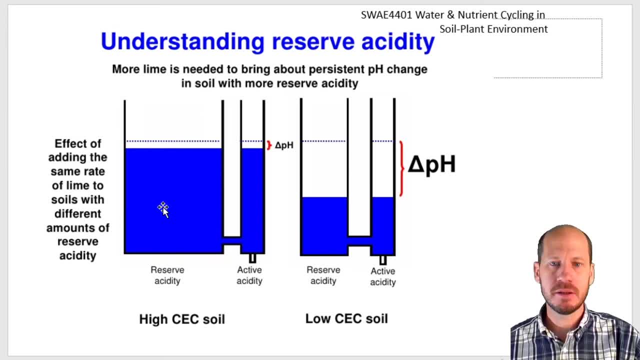 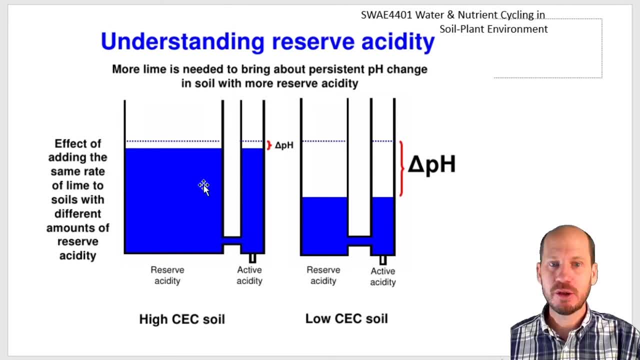 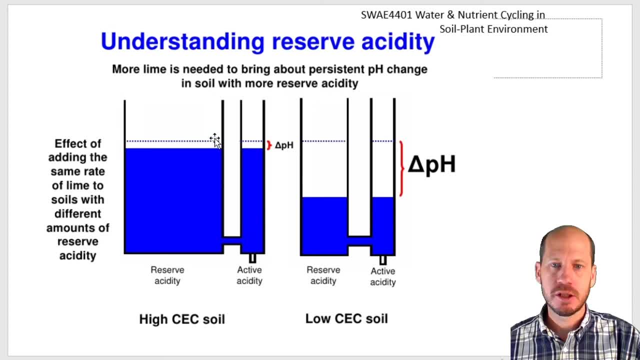 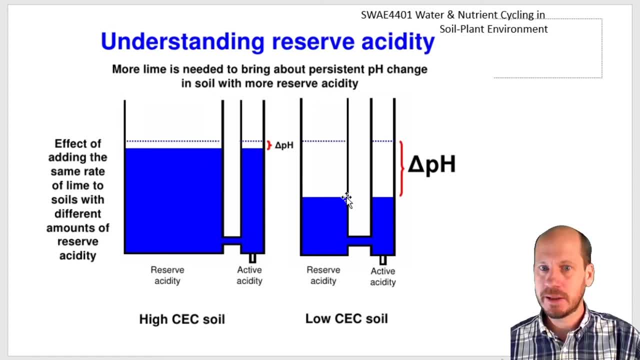 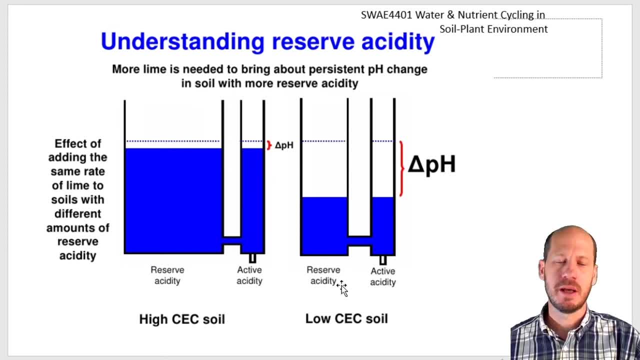 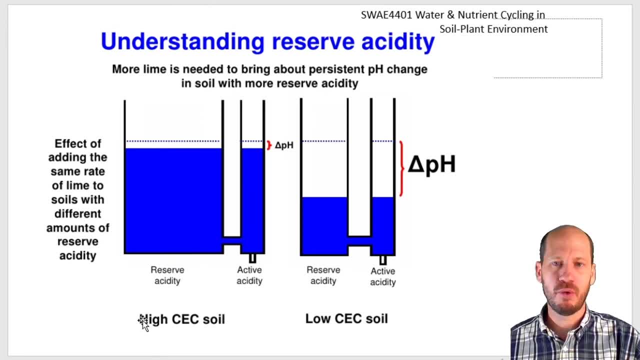 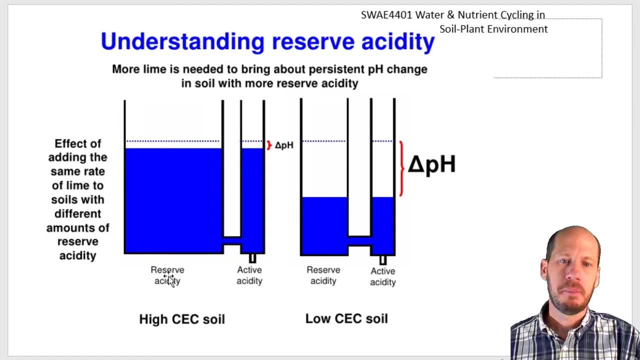 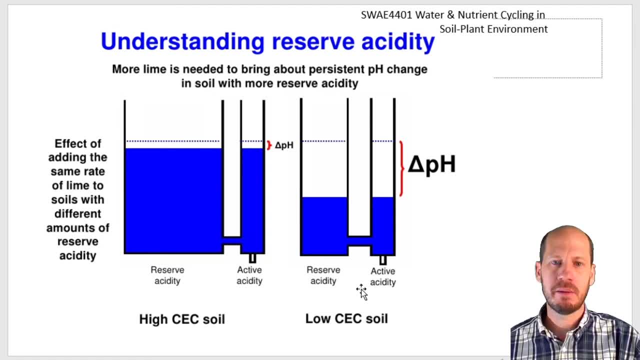 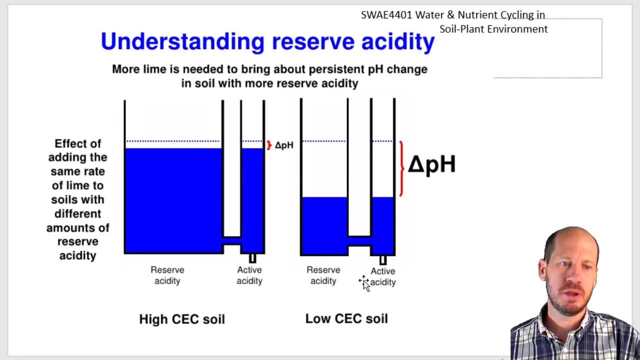 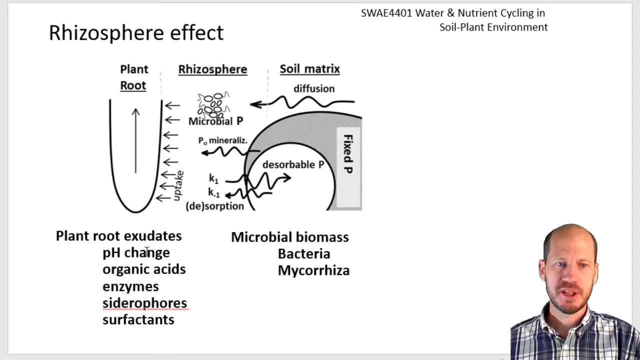 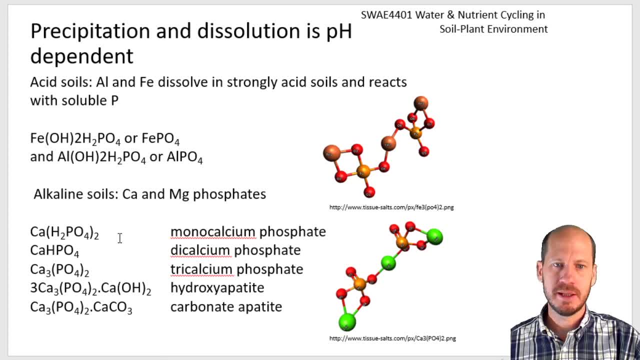 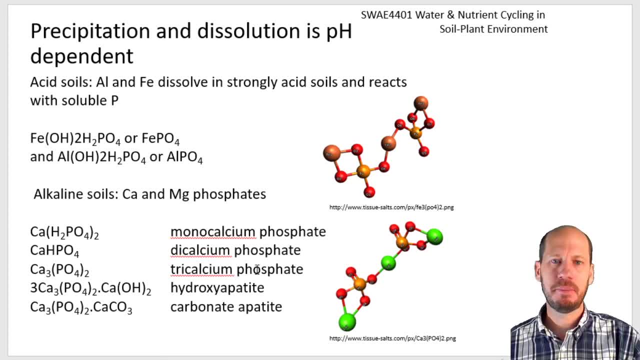 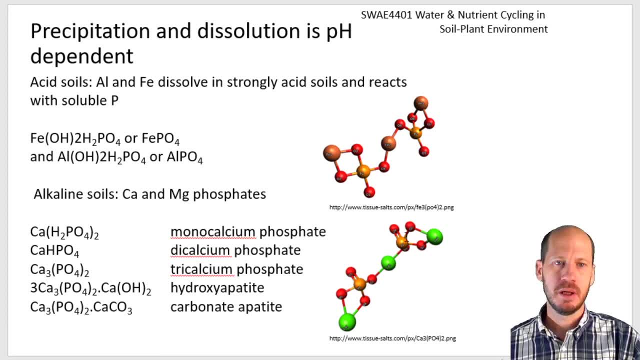 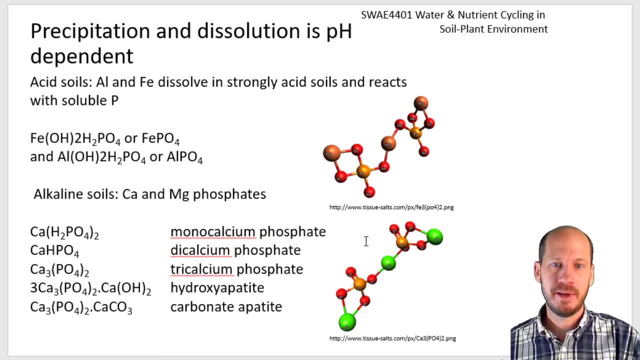 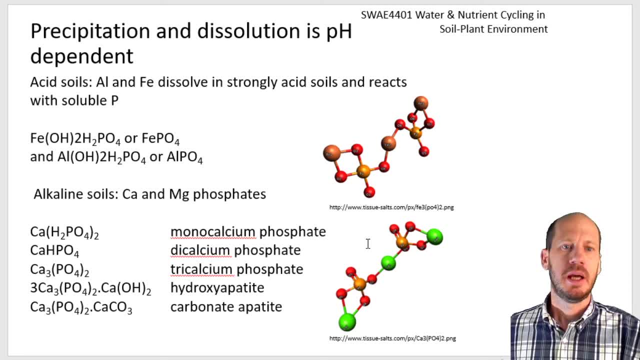 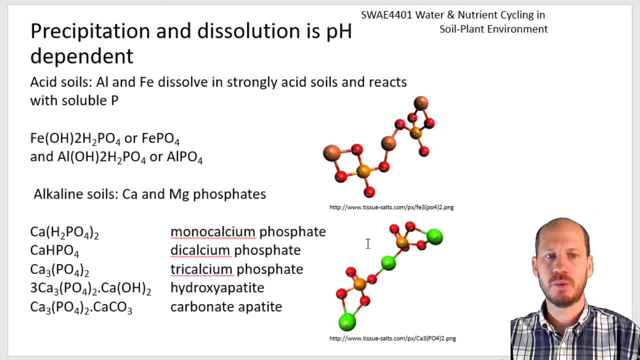 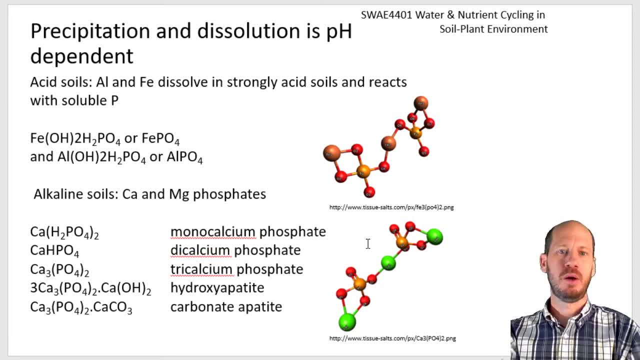 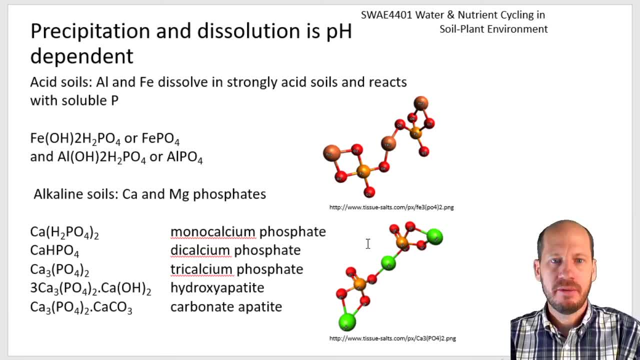 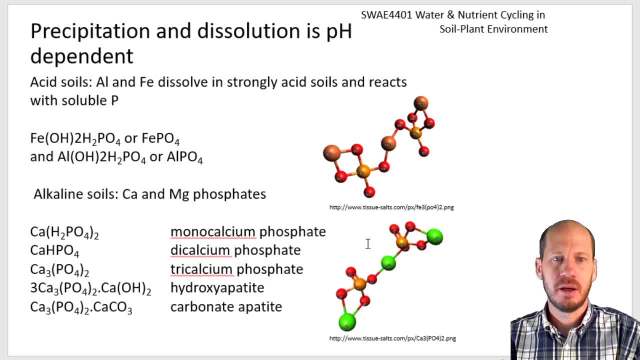 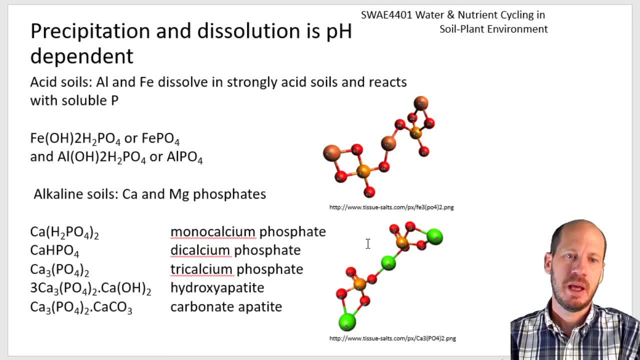 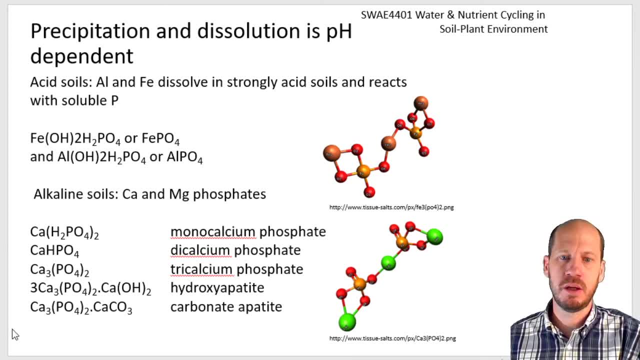 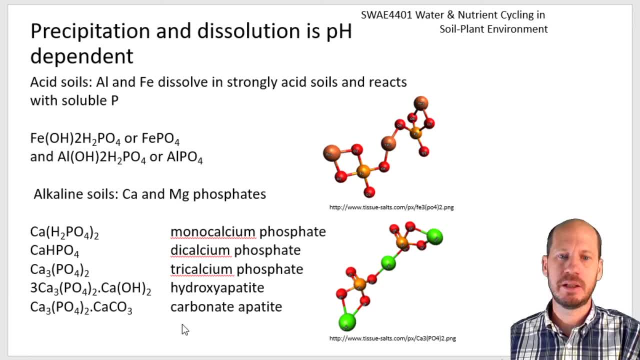 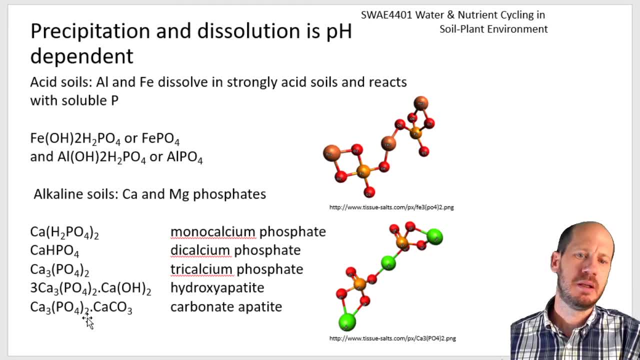 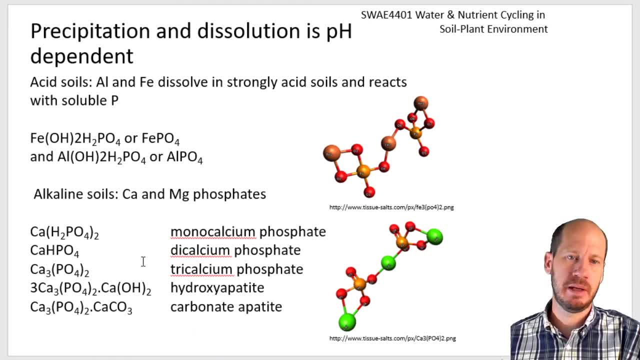 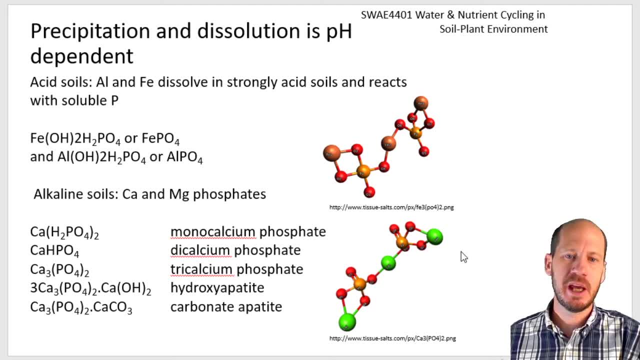 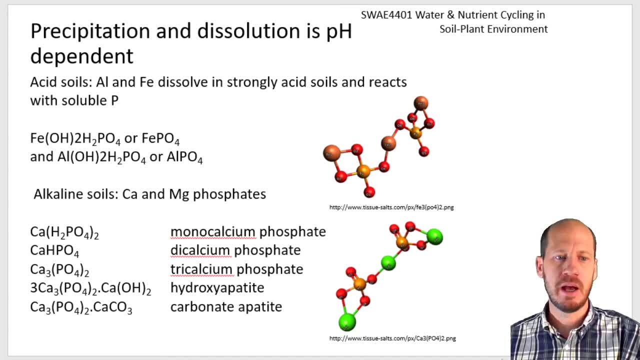 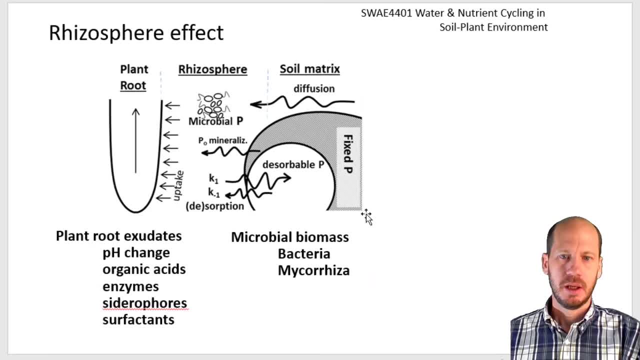 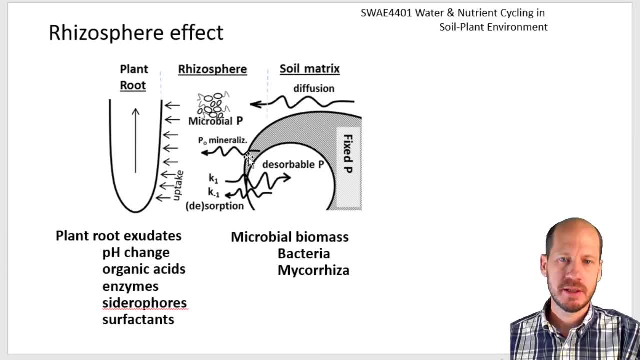 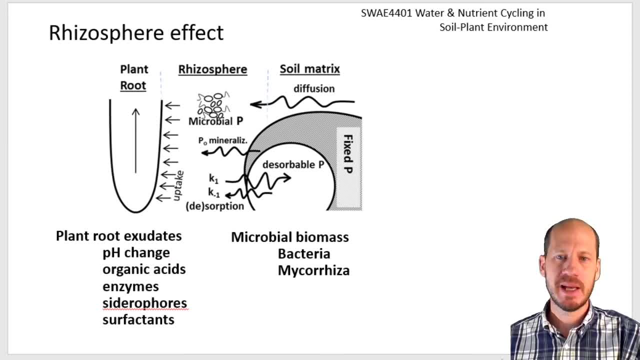 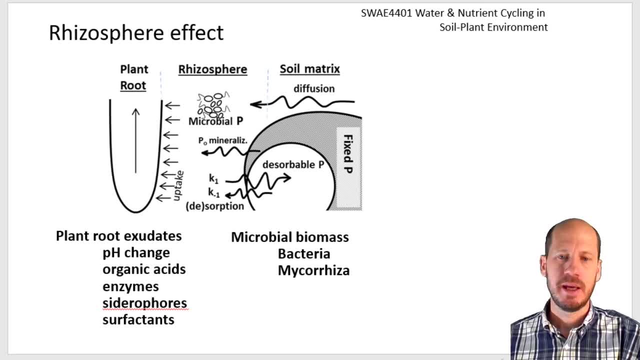 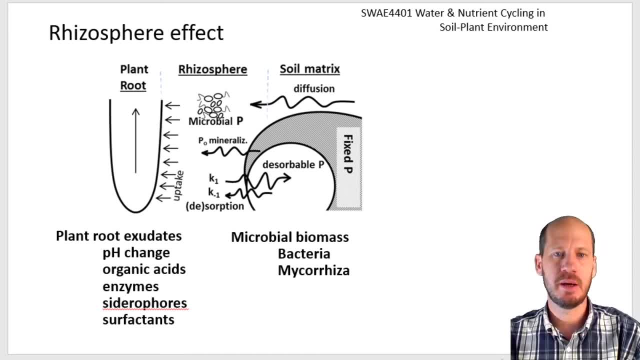 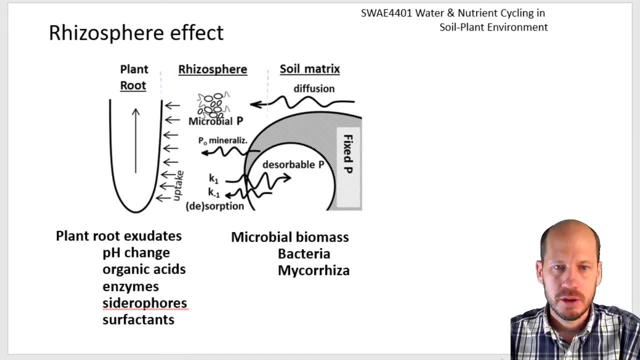 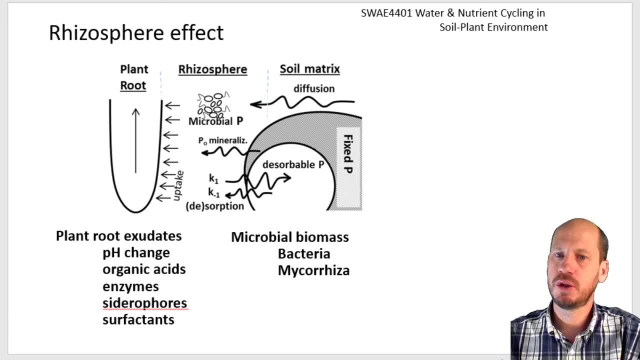 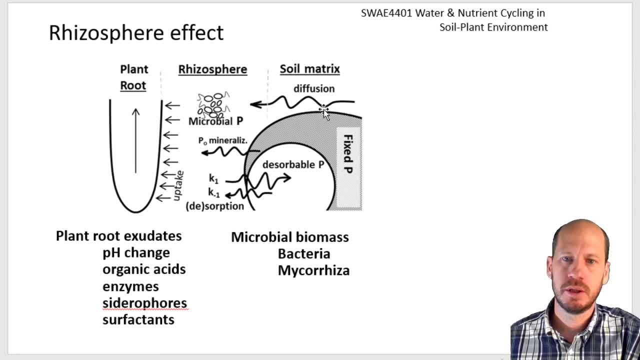 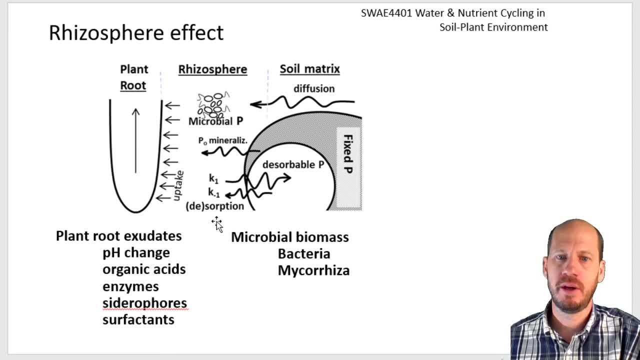 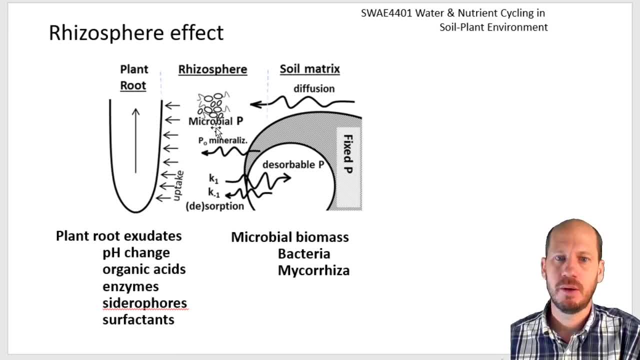 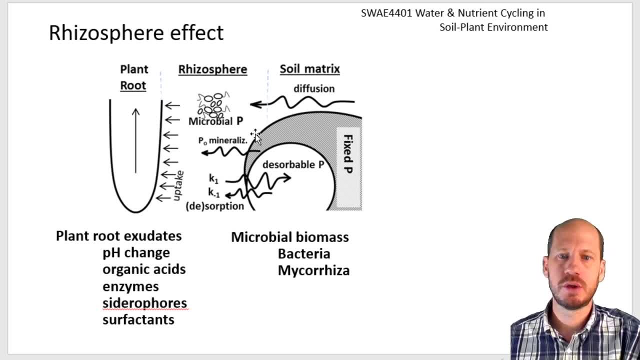 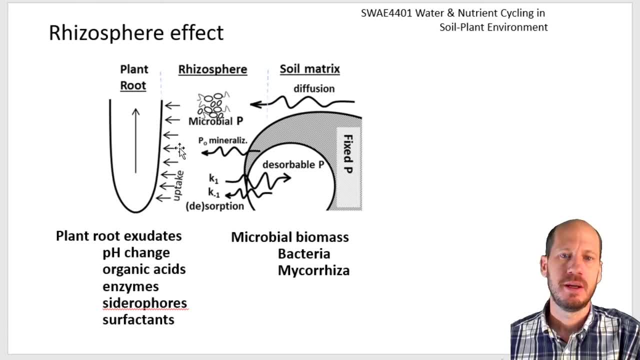 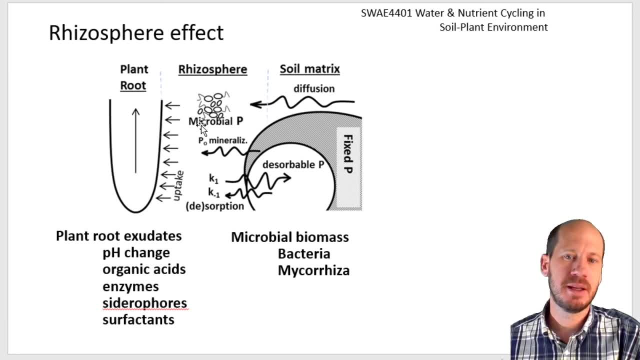 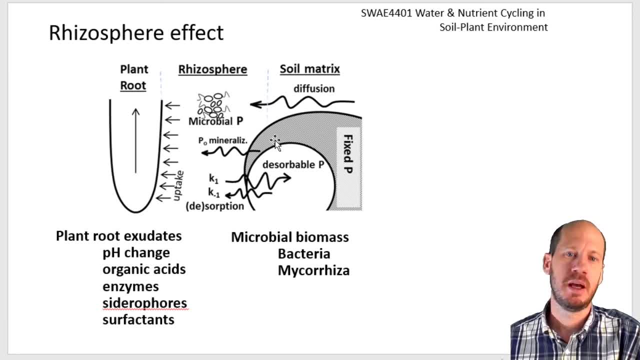 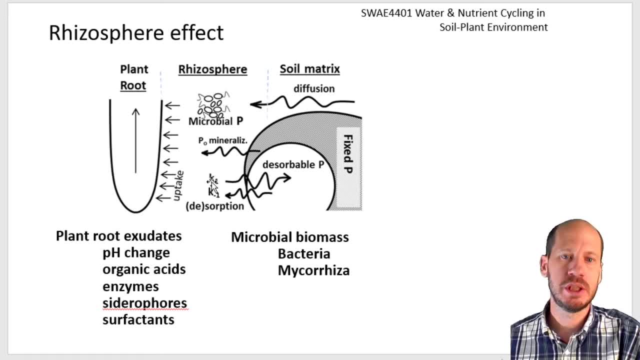 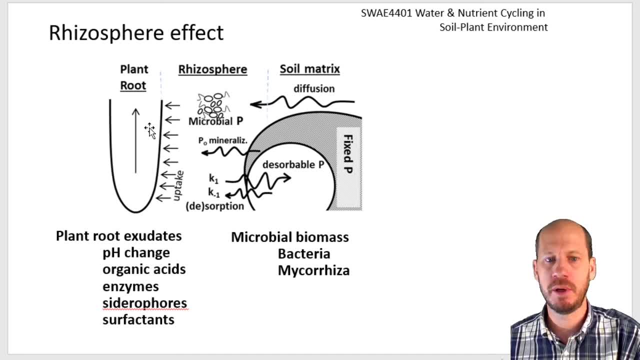 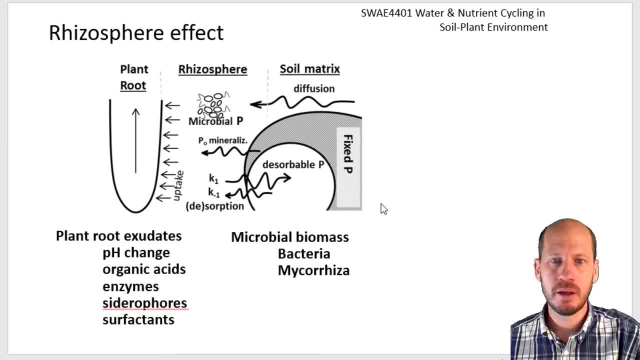 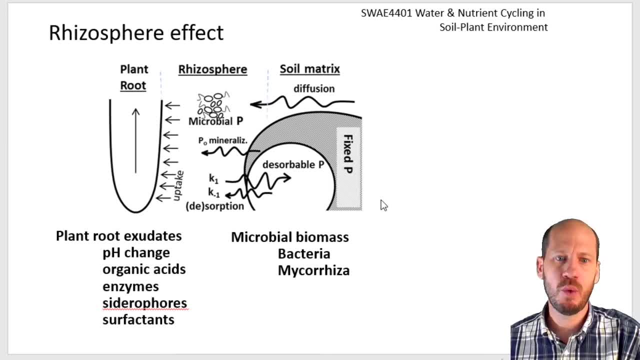 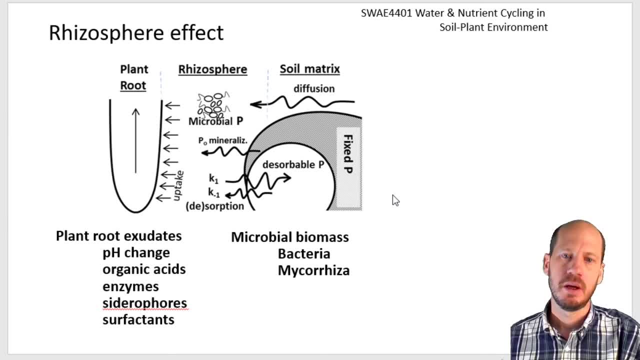 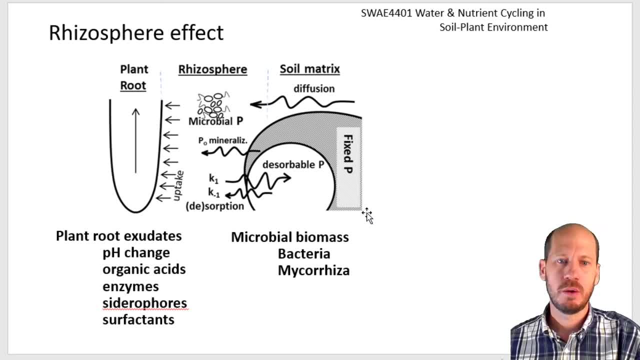 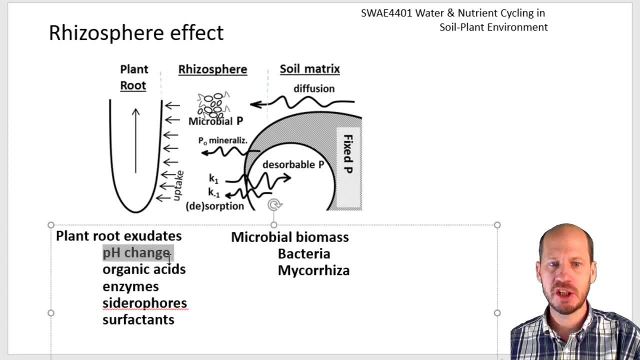 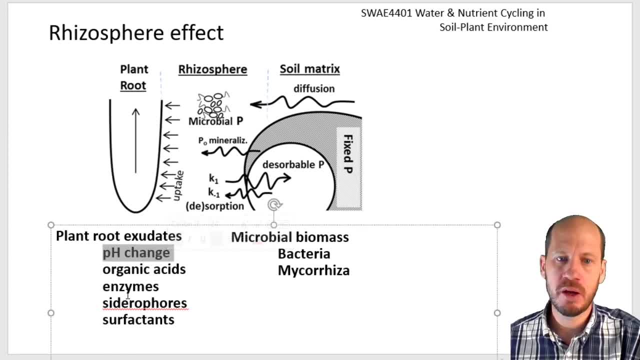 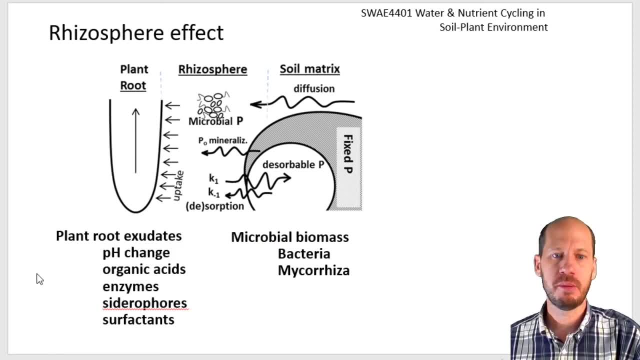 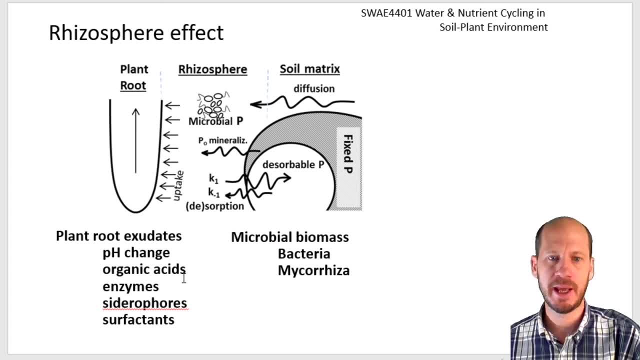 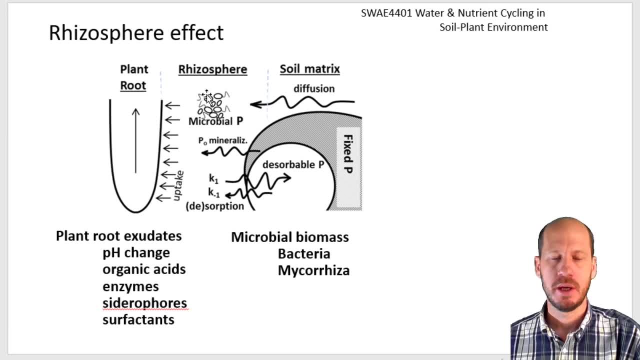 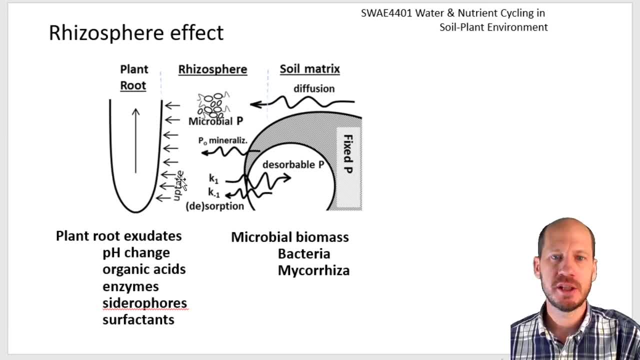 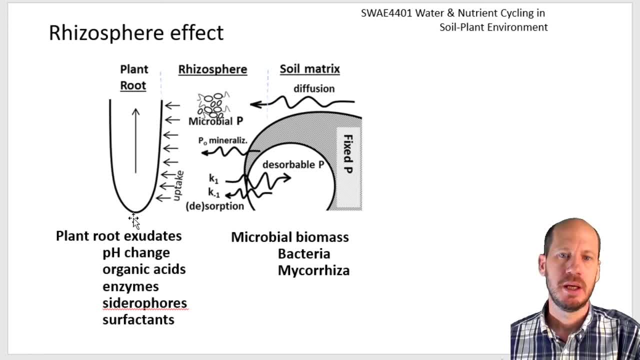 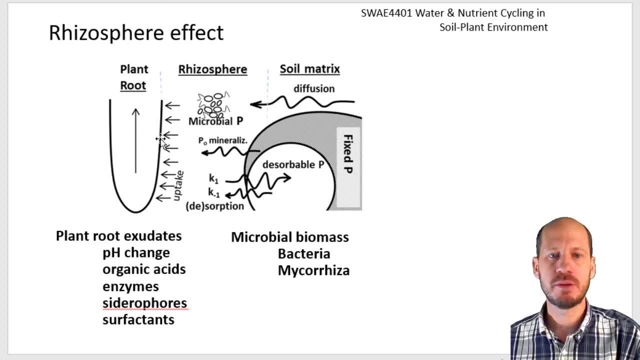 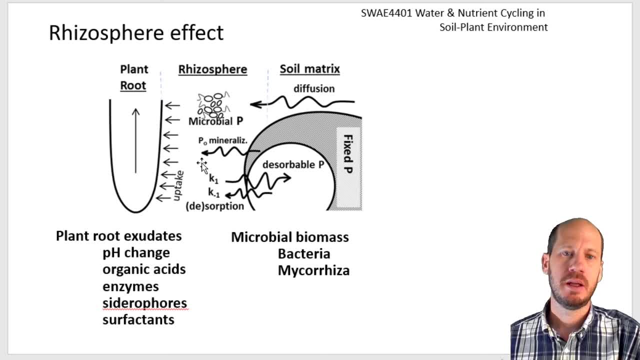 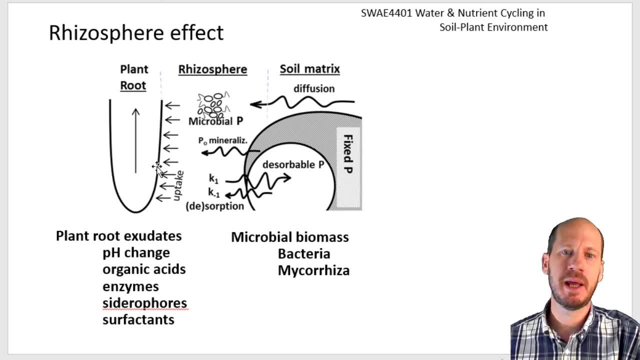 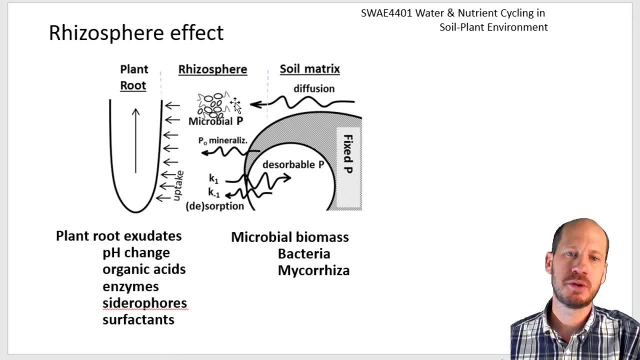 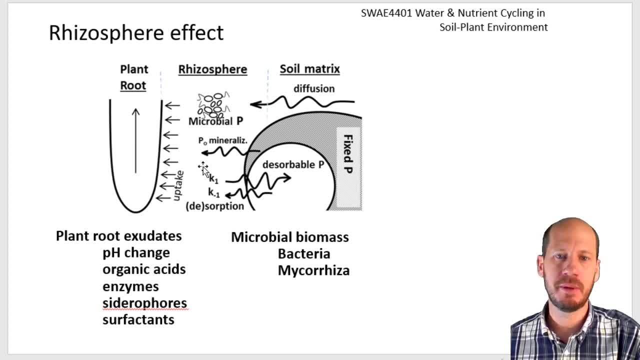 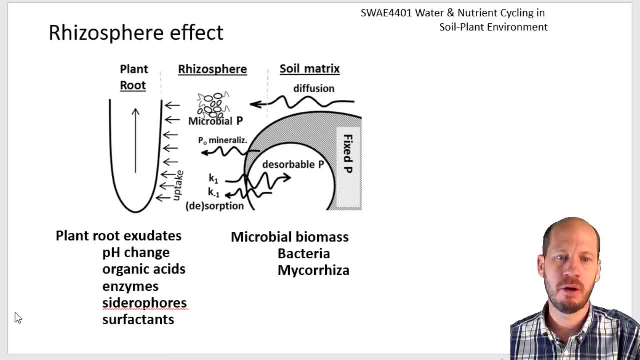 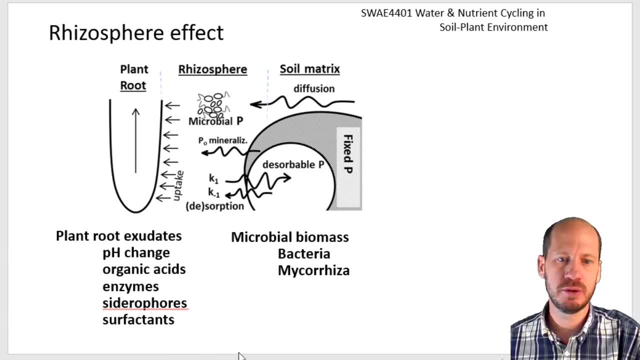 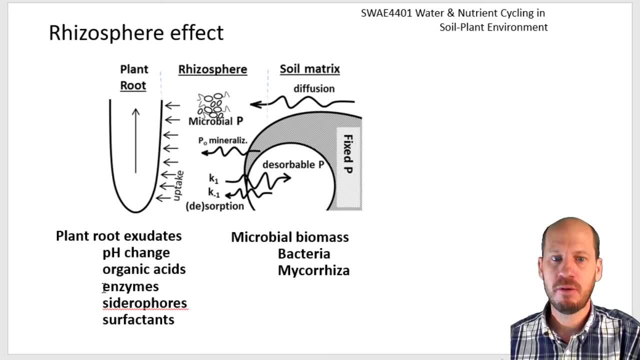 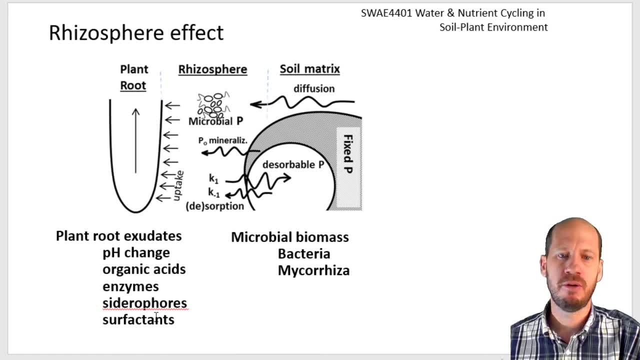 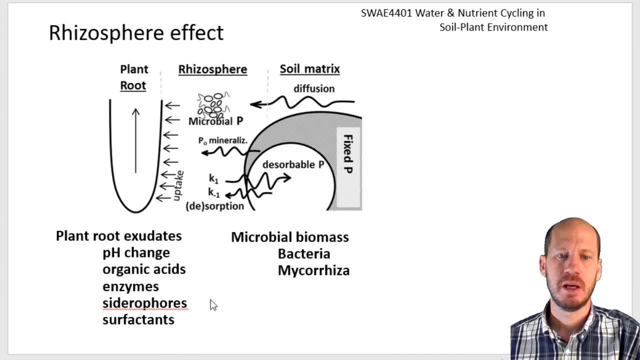 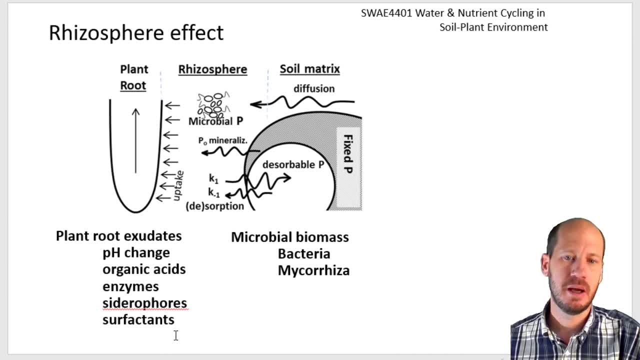 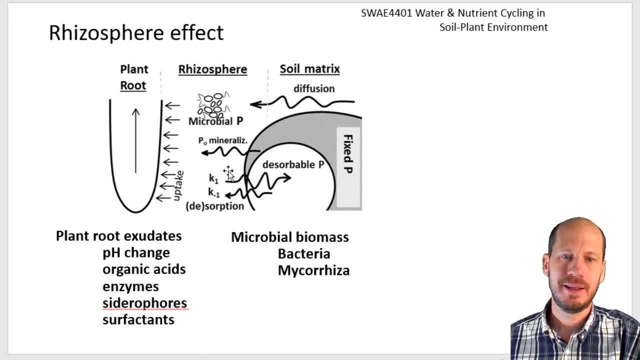 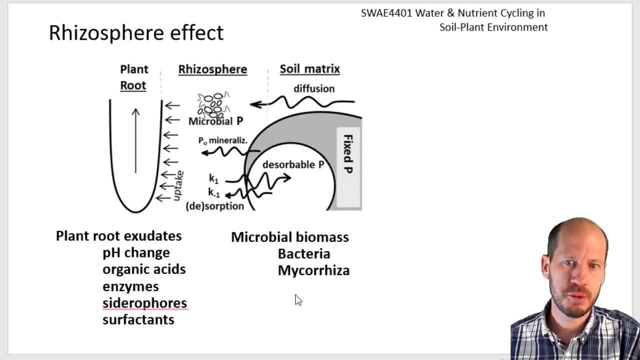 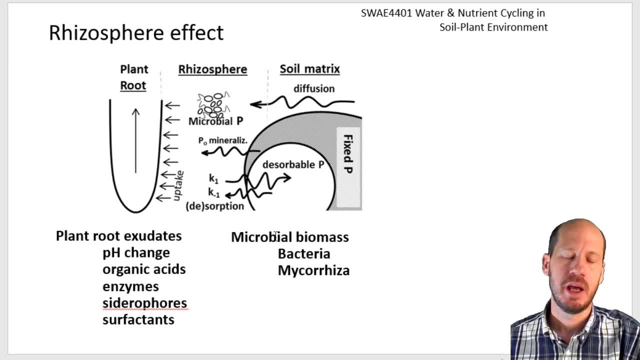 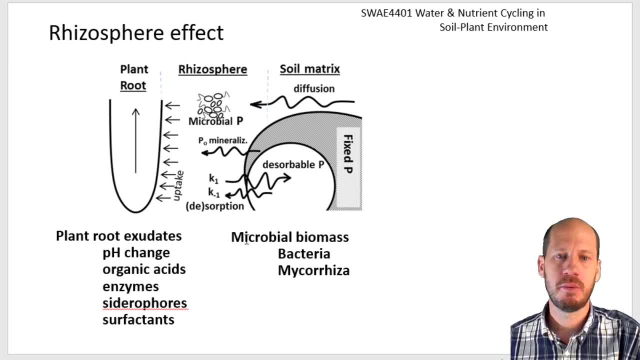 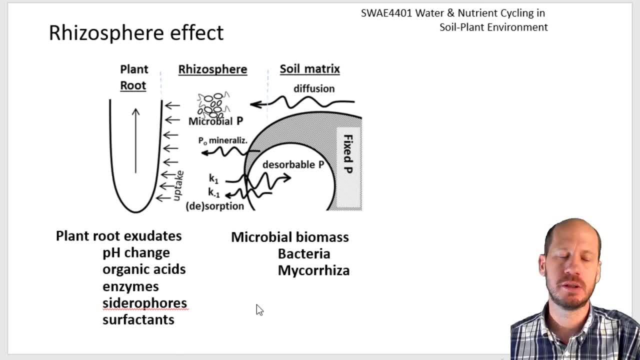 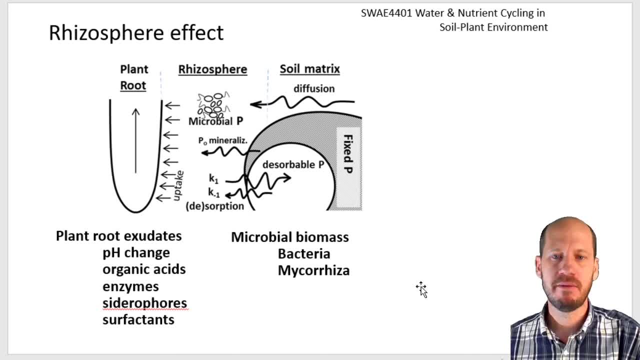 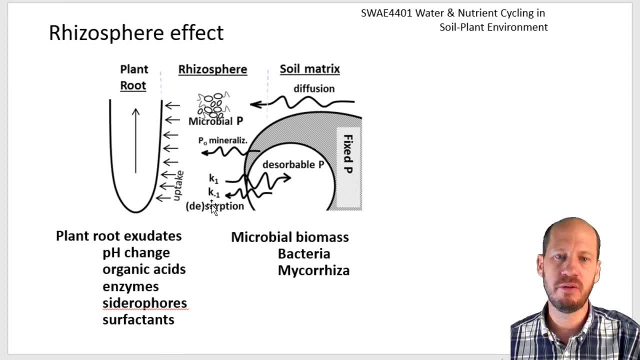 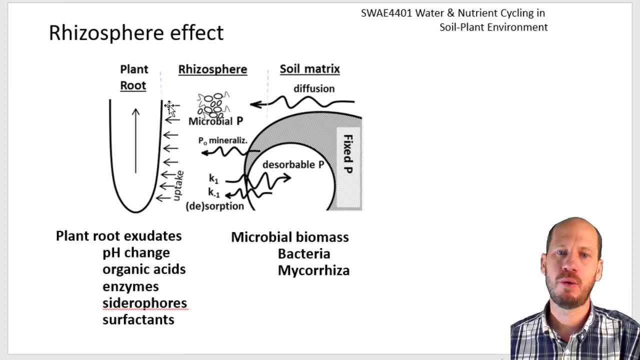 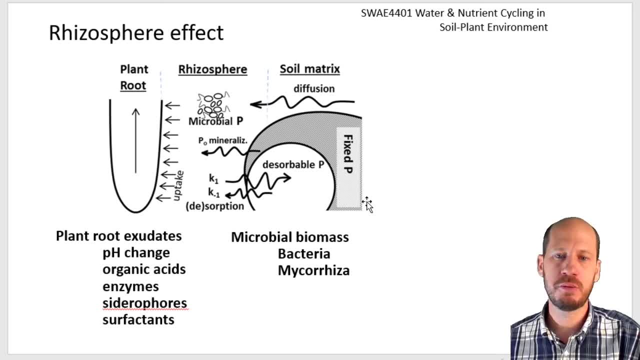 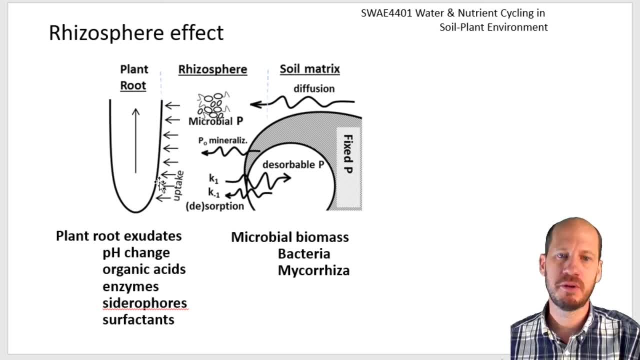 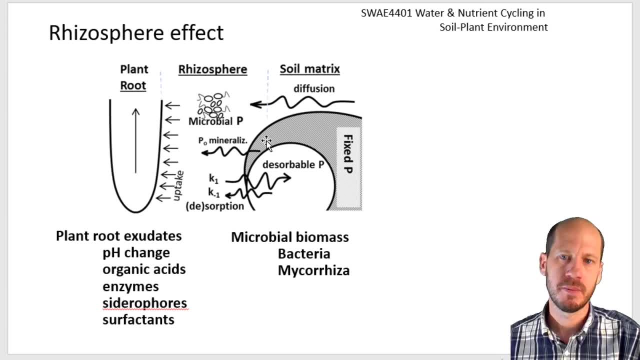 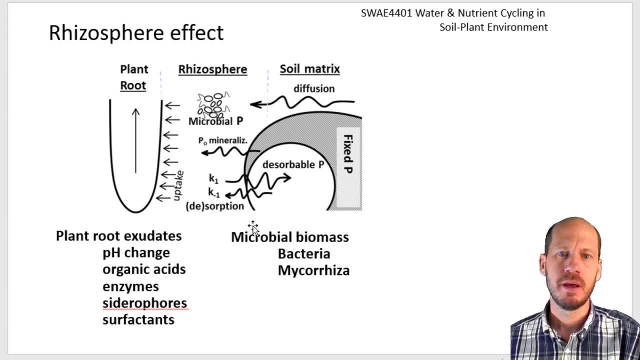 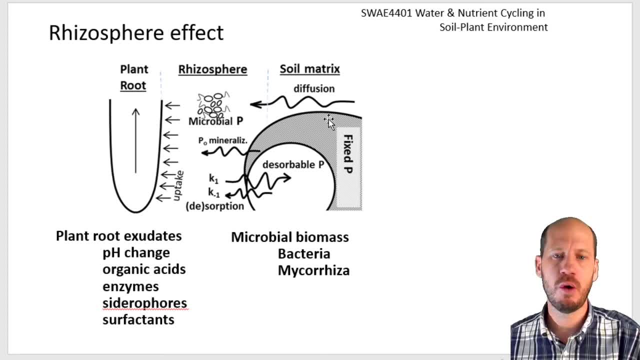 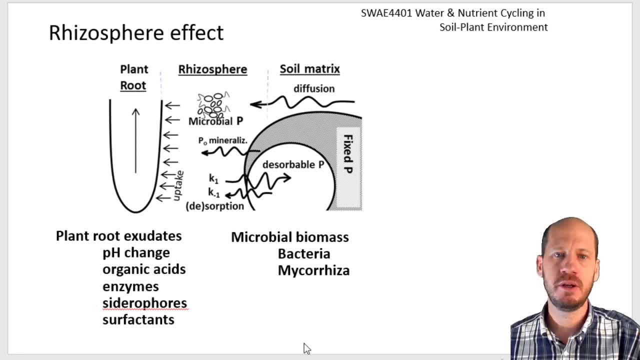 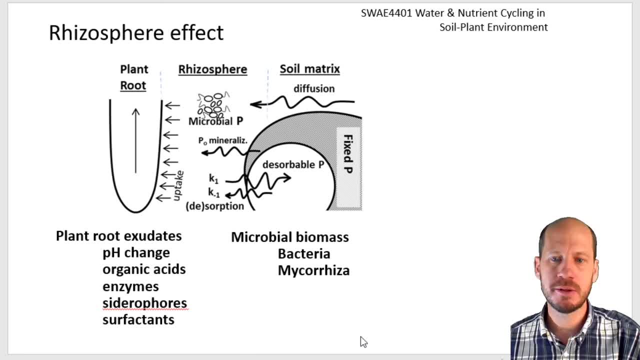 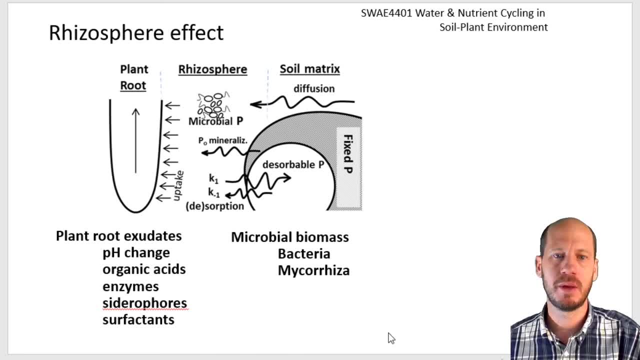 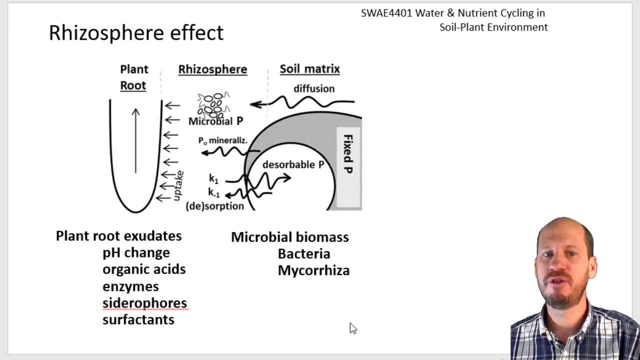 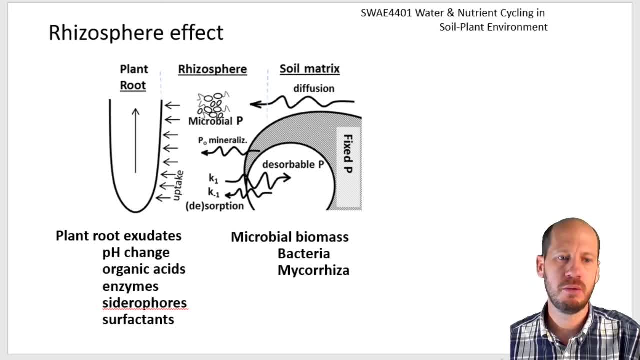 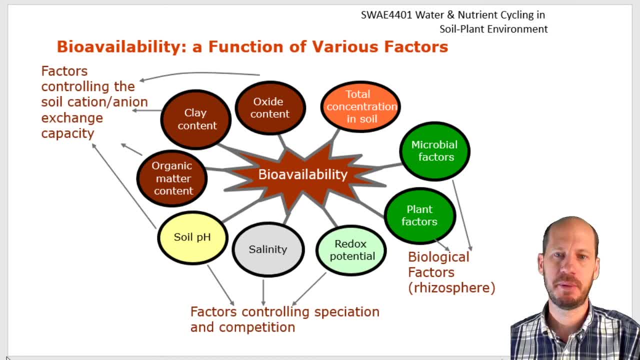 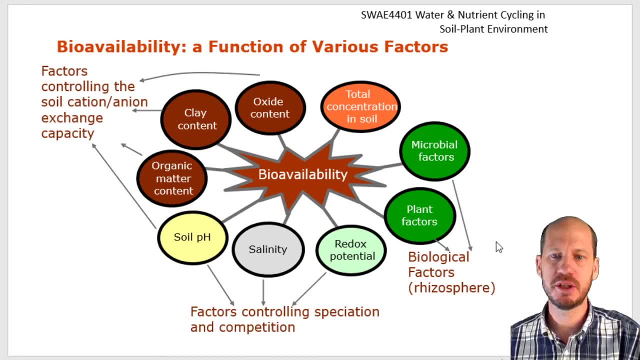 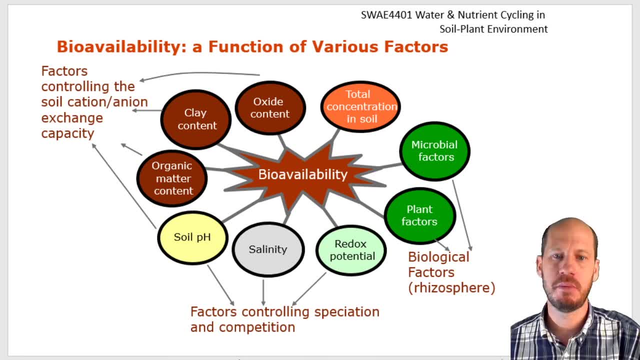 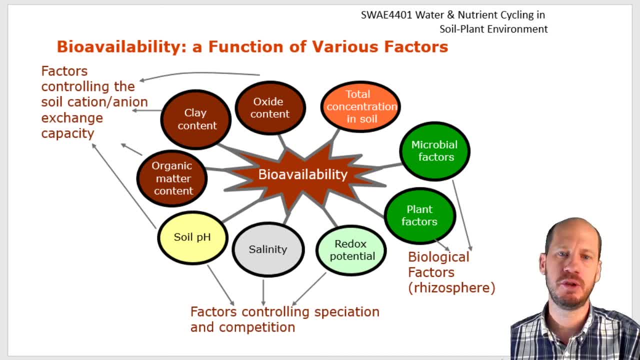 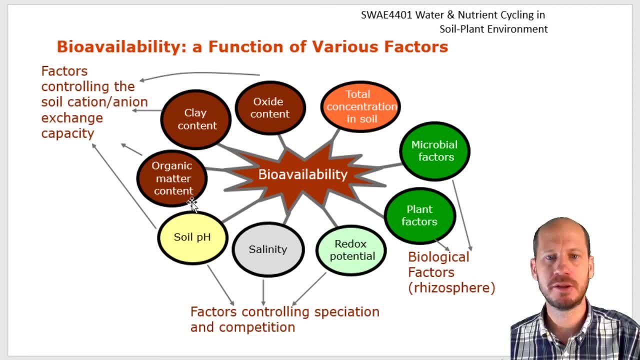 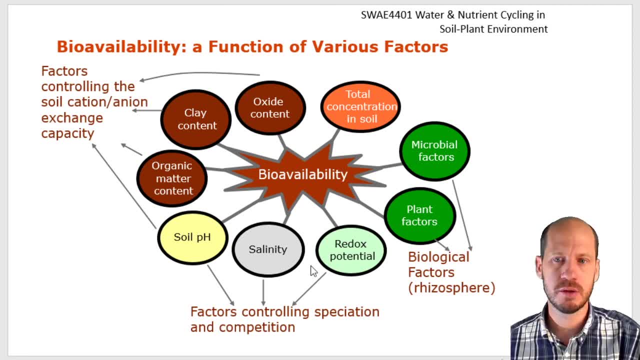 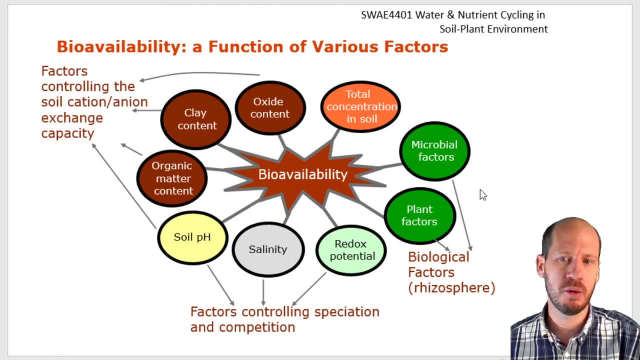 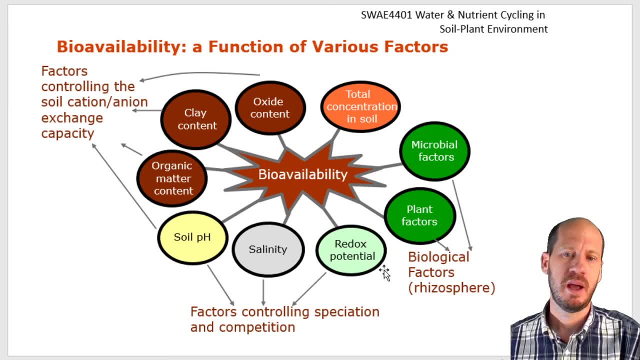